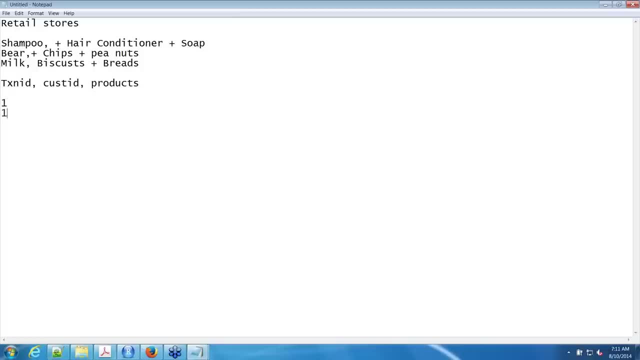 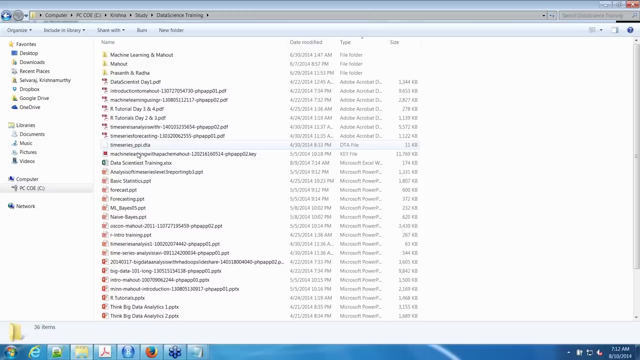 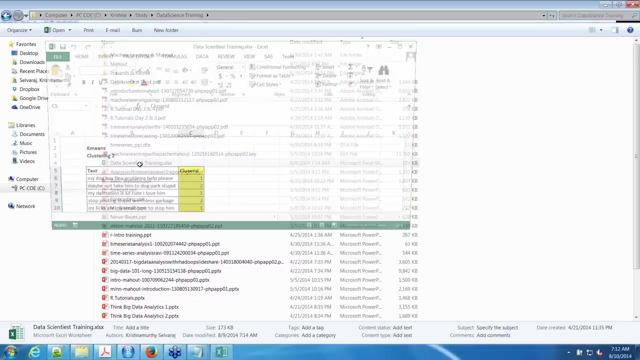 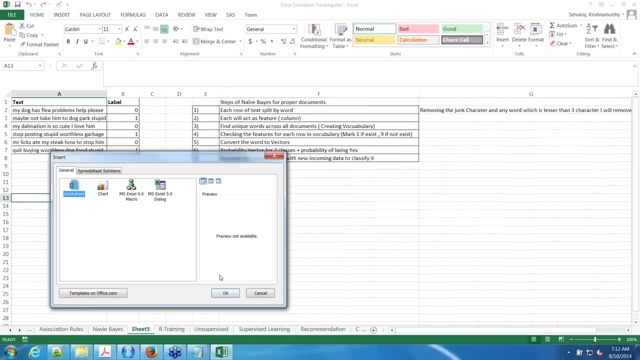 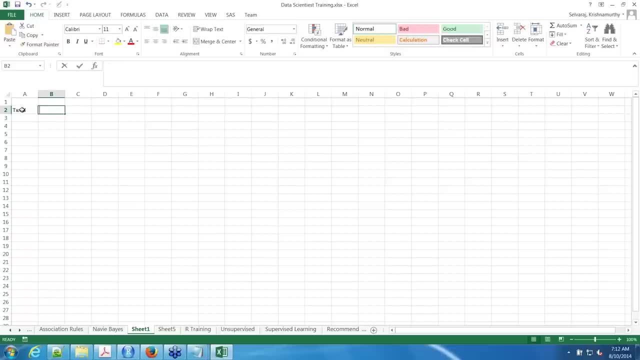 11111,, so designá 11111.. 11111.. products. so same first transaction and same customer say 100, customer is 100, same customers buying different products. so take the second transaction. second customer is buying. 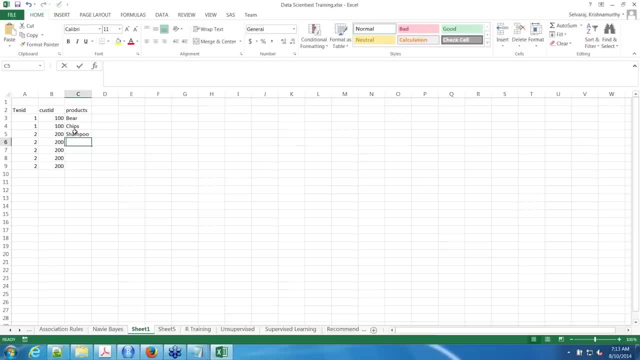 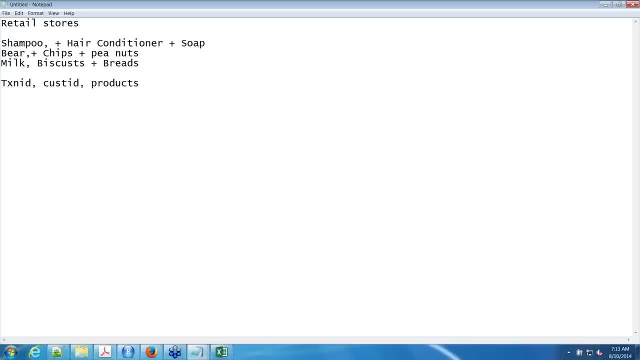 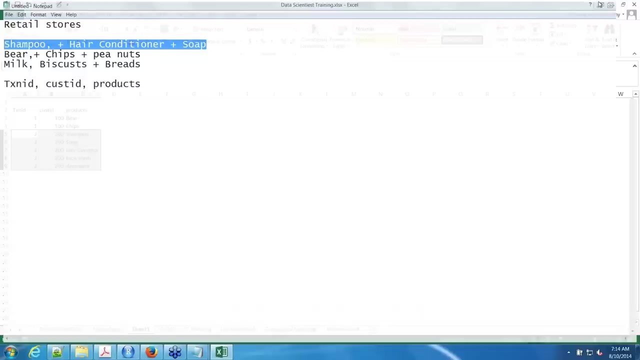 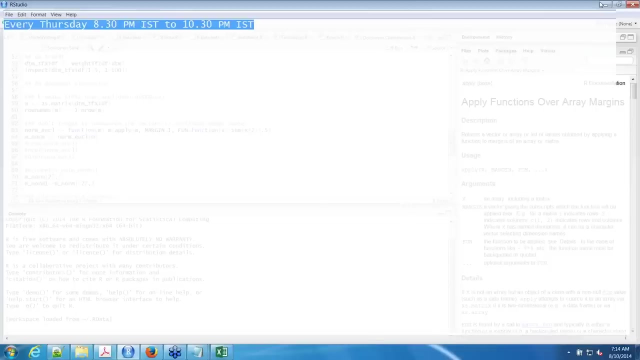 So now what I want to understand. I want to understand what are the products which is collectively and frequently purchased together by customers, more customers. So if more customers are buying a product together of a same product, where what I do is like I understand and find out what is the maximum percentage of level this product. 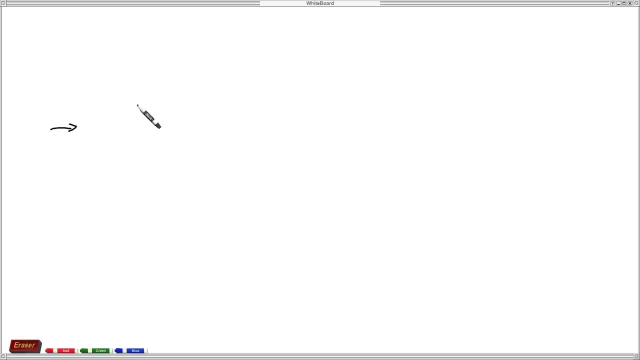 are purchased together. So I have a shop entrance And I have a soap here and I have a shampoo here, So whenever person wants to come and buy soap, he will buy and he will go out of the store. So now, with my analysis, what I do is like around seventy percent of the customers who 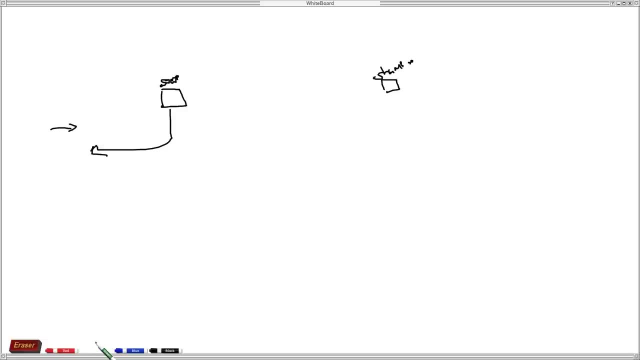 buy soap. They buy soap and shampoo together. So what I do is like I go and place the shampoo over here. So what happens? my intention is to buy soap, but by seeing this, if this is also my need, I need to buy it. I pick up two things and then I come to the counter. 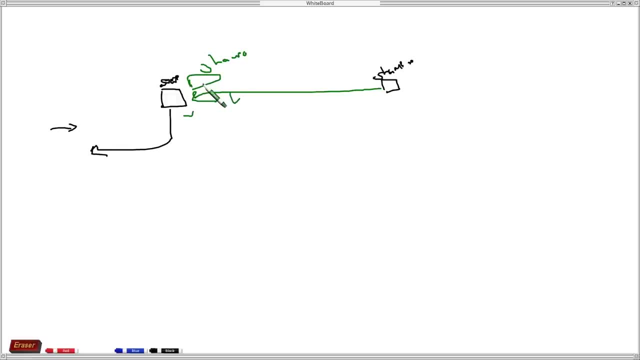 So what does it means is like collectively placing a products which is of similar needs and as well as the customer likings together, So So that one product I will promote which in turn sell two products. The cost for my marketing is one product, but the selling is of two product. 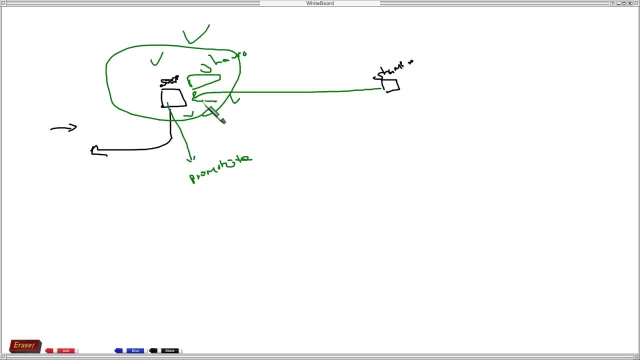 So this is called association rule mining, which is also called market basket analysis. So this will lead into the recommendation of a product. So So, So yesterday I think Asha asked target with this recommendation engine, right, ok, So now what happens? so collectively, I purchased together. ok, sorry, I know it's not ok. 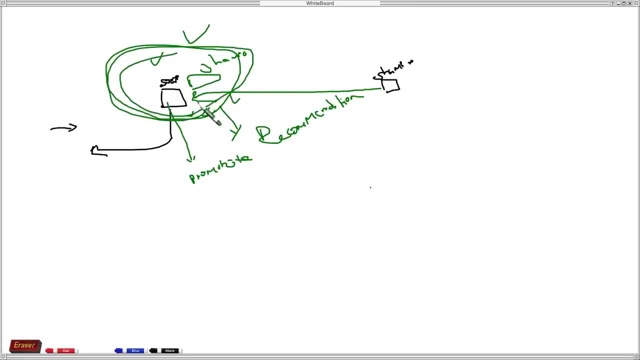 Ok, So what happens is actually products are together, So with this I know the customer id, what all frequently buyed and I profile them. So what is the key part of this? What is the key part of this? Which data is a key? 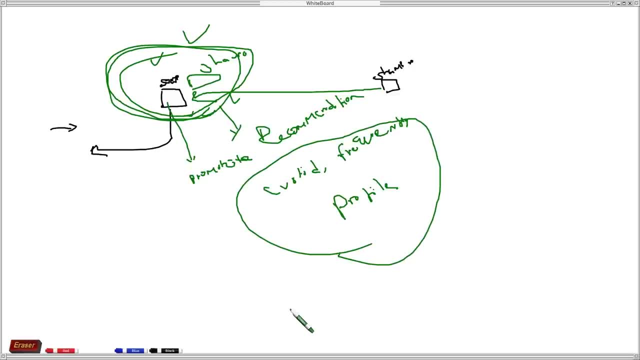 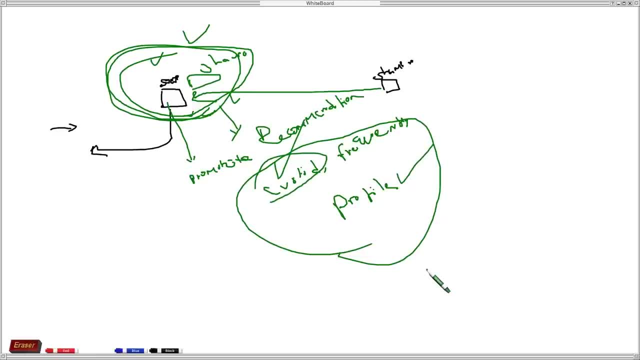 When you have the customer ID and the profile and you can profile. so if you go to the supermarket or hypermarket, sir, can you give me your mobile number please? And they ask while you are standing in the queue for billing. 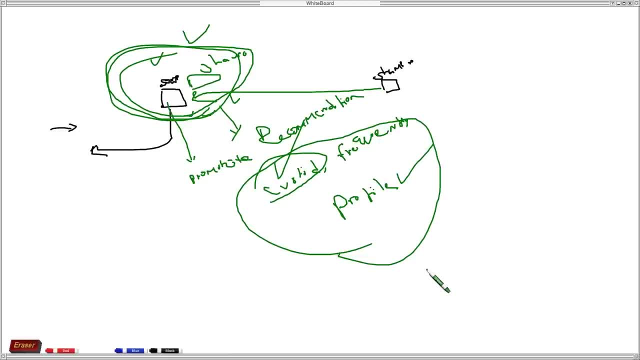 they ask you to fill a form, So its main purpose is to profile them. Once they profile them, they can know what Krishna is buying. what Krishna needs are what he did for last six months when he came to the shop. when he not came to the shop, 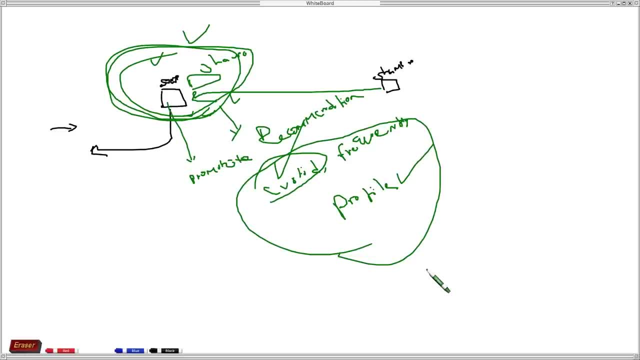 why he not came to the shop. All the kinds of profiling. once he does, that is the biggest asset for retail stores. So, based on the need of the customer and based on his purchase behavior, the products will be recommended, offers will be coming. 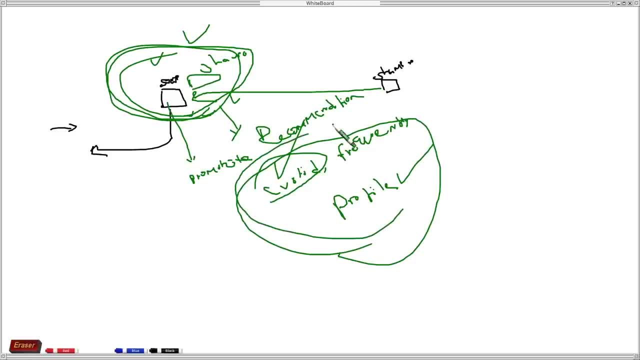 all those things will be in line with the profile, Do you agree? So, based on this, only the target. example: target did the promotions and offers to that particular woman. Is it clear or no? Okay, So in line with the customer ID. 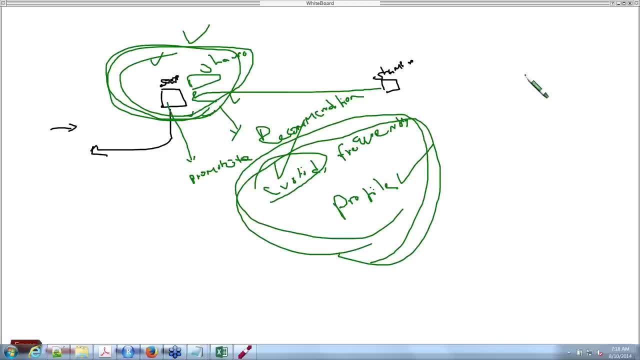 in line with the customer ID. everything is there Now. in India, the retail stores are biggest in demand and, as far as the data science for retail stores are highly paid. Why? Because of the upcoming of online stores. So now you can buy the groceries in online. 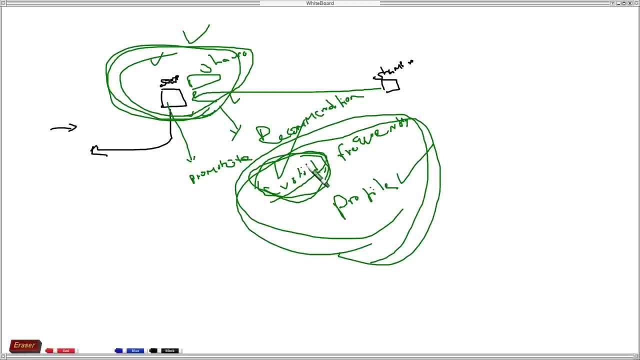 Everything you can buy in online. A lot of people buy in online. The retail stores are just they have less kind of profits and less customers and they want- they want to market it more with a lot of offers so that they can compete with the online and as well as they can sustain the market. 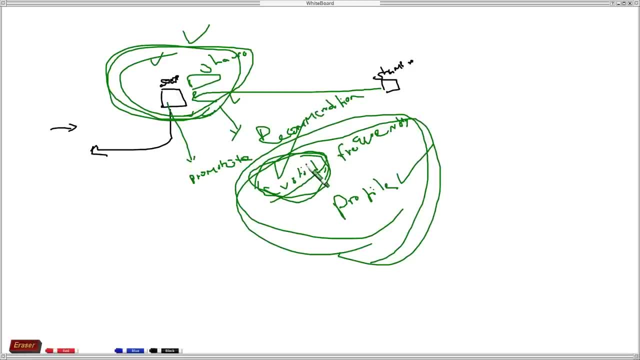 So that's the reason- a lot of MBA guys and as well as in combination with the data science guys. what type of change you can bring to the retail store so that attract my customers to come to the store with it and purchase the things? 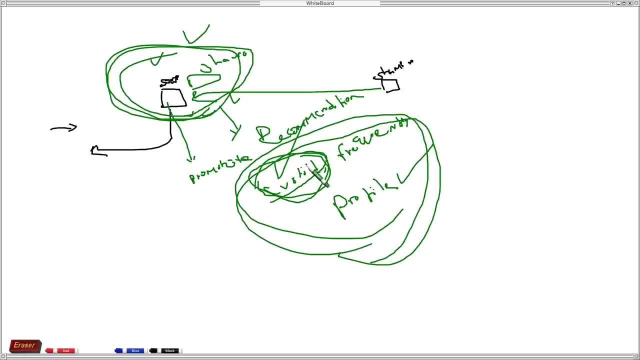 Okay And purchase the things. So all this is a good kind of a success, A good kind of a sign where you can bring some new kind of a dimensions to the retail stores of promotions, recommendations, offers to make the customers to come into the stores and buy. while buying, the biggest asset is going to be the customer profile. 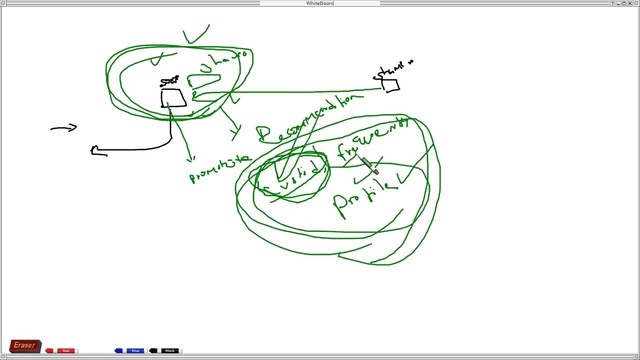 Once you profile them, you build anything to that you can easily market to them and make them to come into the stores. Then whether they purchase or not is a different game. So that is called association rule mining, which we are going to see how. what are the products which is frequently buy together, which helps to promote one product, and try to market by keeping all the products together, which is relevant, which makes the customer to buy the similar products. 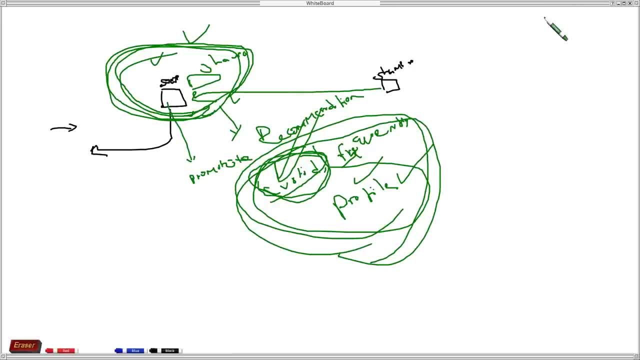 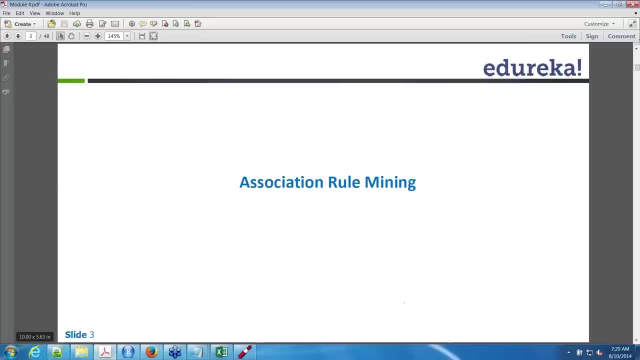 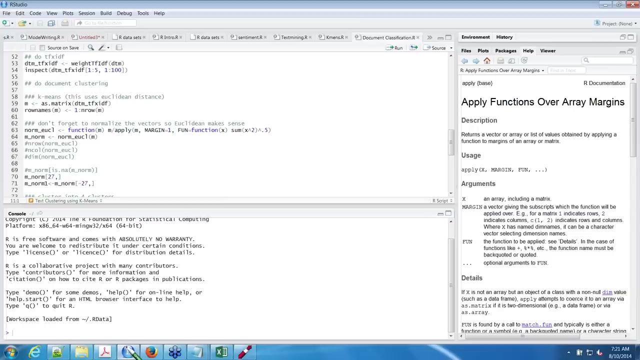 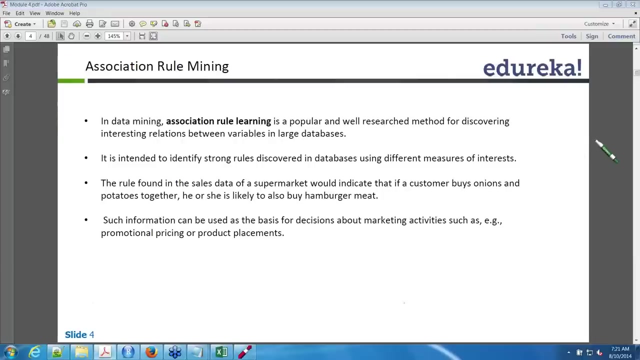 Got it. Is it clear what we're trying to do here? Any queries on this? Okay, Good, Okay, Good, Fine, so it is one of the very popular method identifying a strong rule discovered and between the products and between the different baskets. when you say different baskets is equal to. 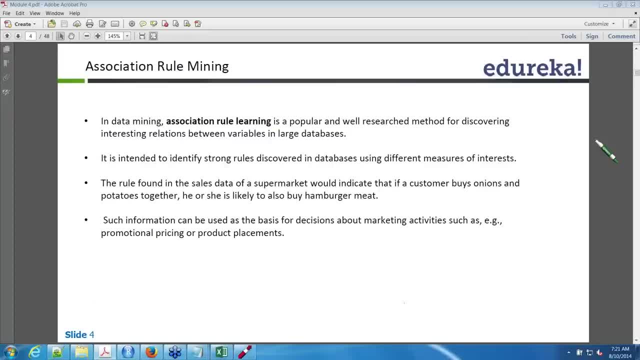 different transactions. So this is some of the examples: when customer buys onion, buys potatoes together. So all those examples of what we have seen, and with this we can make a kind of a set of rules which all the products to be combined together while placing in the stores. 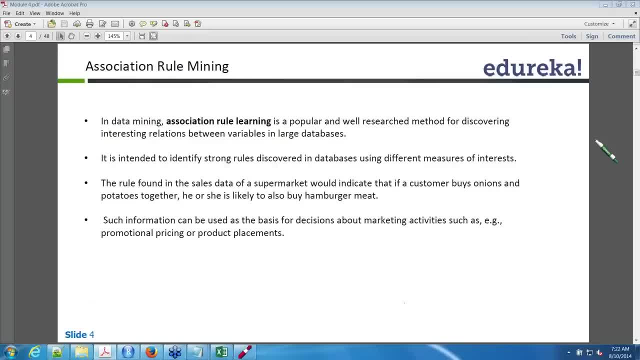 If you look at the bill counter when you stand for the bill. So especially in Total Big Bazaar, where the chocolates and the batteries razors all are kept near the billing counter. is there any specific reasons? Essentials and attract children's shells face. okay, okay good. 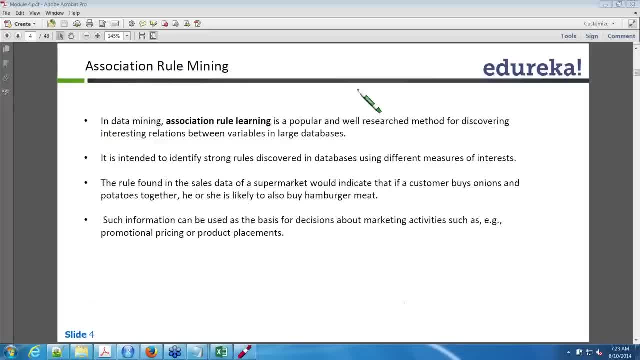 So it's more of essentials and attract children's. while you are standing in the queue, the children's will ask for chocolates and it is in another kind of a sales Okay, Okay, Okay, Okay. So that is the reason, and while you are standing, you might forget to buy the small, small things. 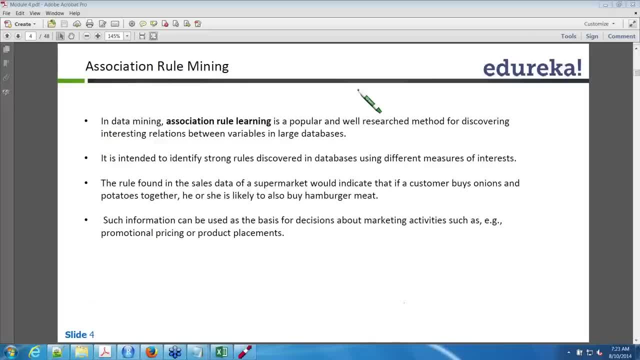 While you are standing, you will think and see all those things which you feel is required. It's my essential needs, So that's the reason it's placed near the billing counter. Yes, Bazaar, good, Good Anup and Bazaar. 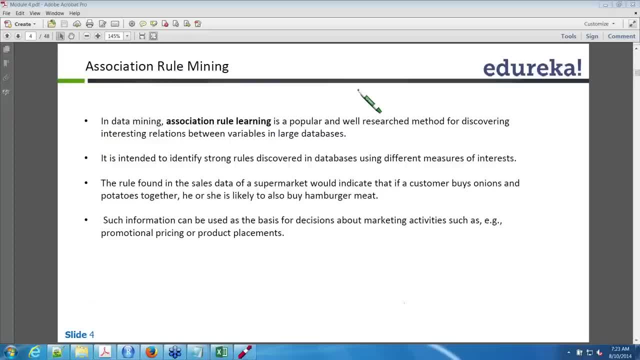 Okay And good to them And in hypermarket if you go. So there is shelf will be there. ground shelf, that is, the racks above racks and above racks are present And the vendors. to place the product in the first rack is costly than the vendors to place. 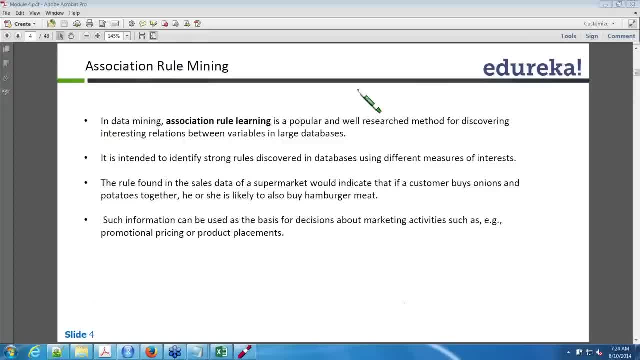 in the bottom rack Any reason? Okay, Okay, Okay, Okay, Okay, Great, Any questions? Okay, Okay, Absolutely. And for a vendors, if they have a presence of webinars, the product the first rack is costly. run the bottom rack. 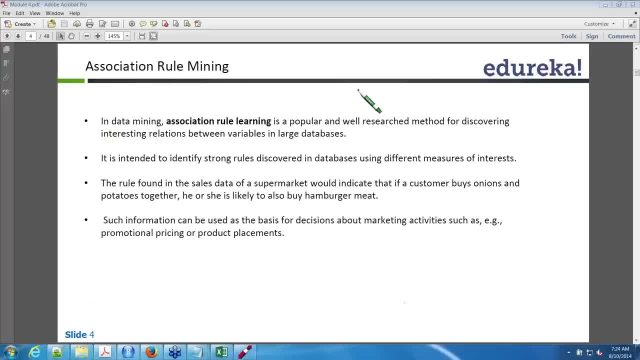 Okay, excellent Catches: customer retention, a standing. we'll have a better look at first track. The chances for the last one is leading proximity at the level of five. Easy, Yeah Yeah. fair point: Fair point: Yeah, Yes. 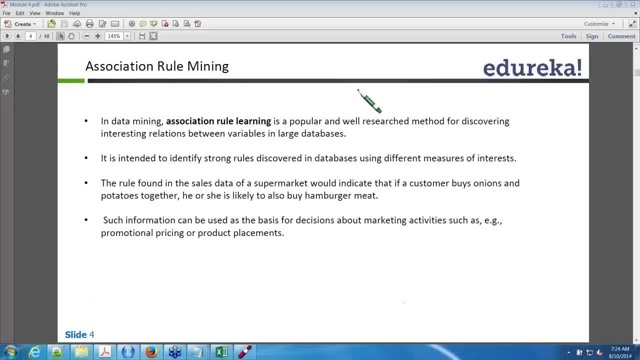 Yes, Yes, Two after. So why? because the point of sale for the product which is present in the first rack is higher than the point of sale for the products which is present in the bottom rack. So that is the reason it is costly. 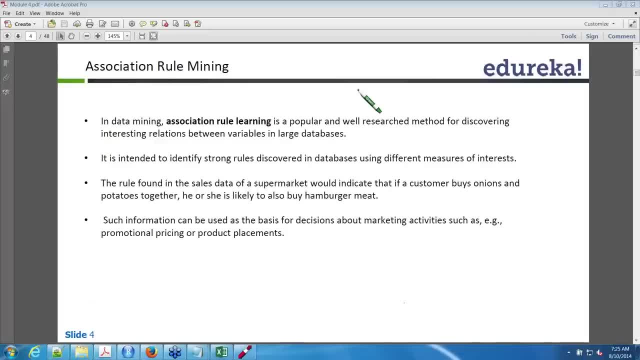 So all this also is a point of kind of a data science, where which of the products can be placed at the top and which of the products can be placed at the bottom, at the middle, So which promotions you can make to make a better sale in the retail stores. 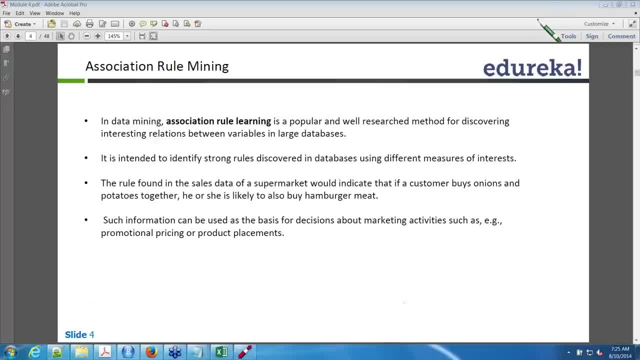 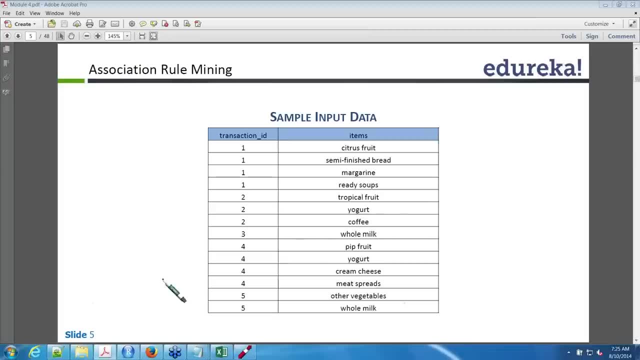 So those are the key things. So now we will get into this association rule mining. So this is the sample input data. I have a different sample with a small set of data. So by the concepts, everything is same, Whatever you apply to a large volume of data. 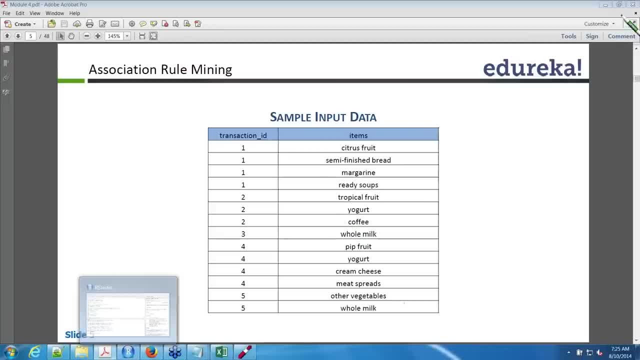 And small volume of data. it is going to be same, And I had a question from Asher: What are the different projects or example where we can use association rule mining? Ok, good, So association rule mining is a better fit where all you have a transaction and where 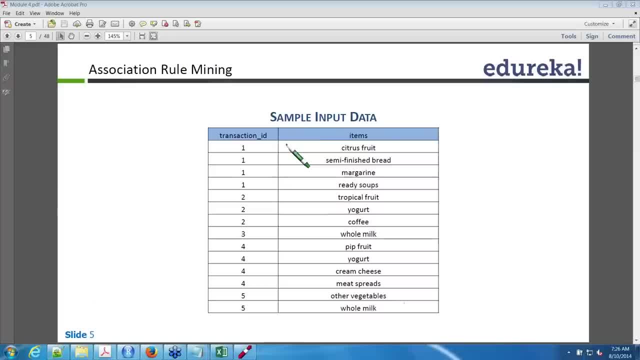 all you have a kind of a purchase or a consumers, You can apply the association, So the majority of use cases. this has been applied in the retail industry. that too with a specific to stores. So if any questions, this is really sorry. if you don't mind, can you please repost it? 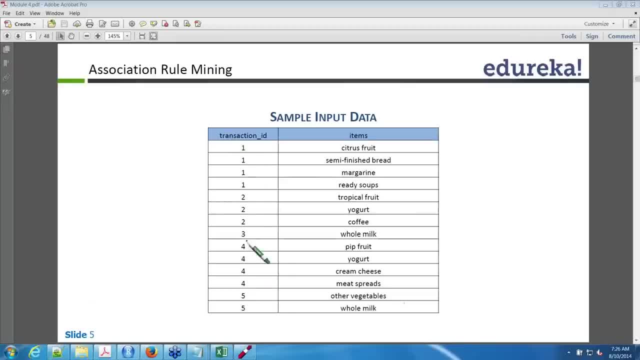 Ok, So if you look at, this is the transaction ID and the items purchased together. So the basket model is comes from the transaction. So in a single transaction, what are the products purchased together? So in a single transaction, what are the products purchased together? 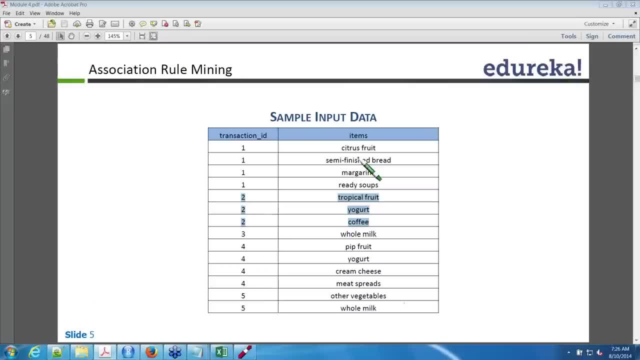 If you look at here, citrus fruit, semi-purchased bread, margarine, ready soup are purchased together and similarly for transaction two, this was the product purchased together. So I have a many transactions and each transaction is going to be equal into a one basket. 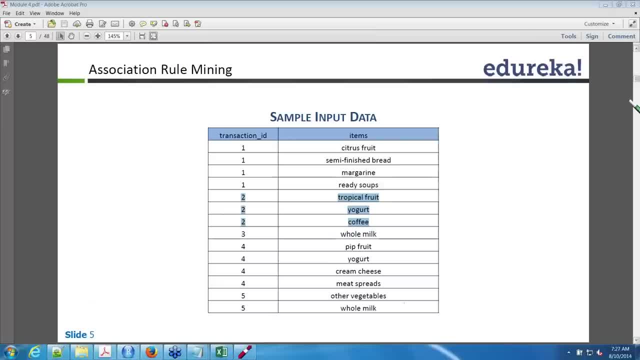 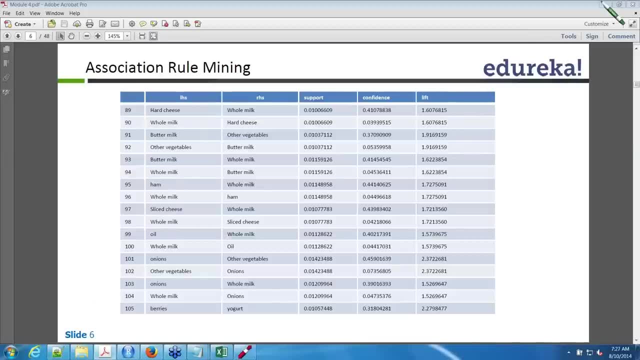 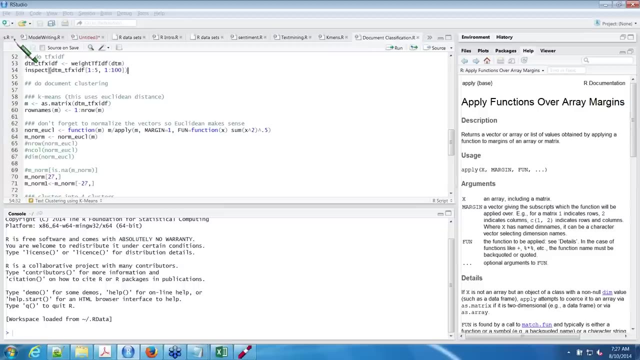 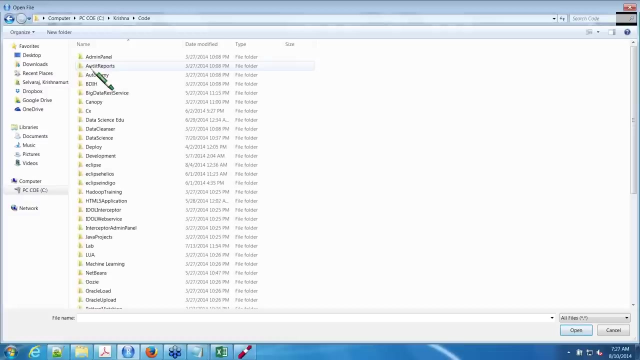 So that's the meaning of it. Ok, So let's go to basket In a basket overall the purchase product purchased together. Hi, mother, Ok, So now we will go and start working on the practicals You want to delete. 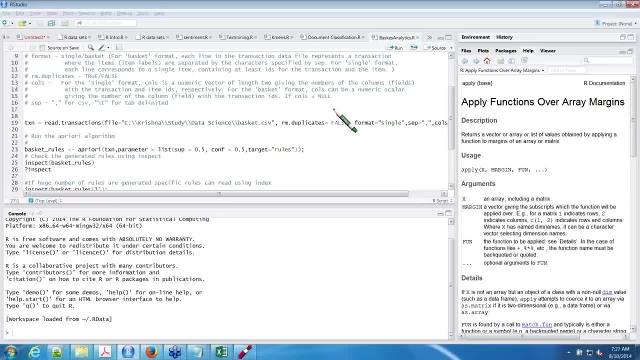 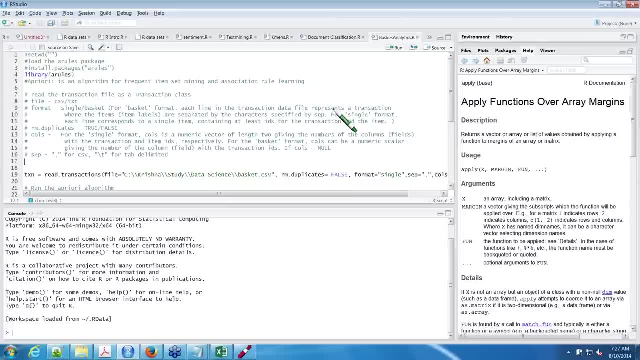 Ok, So it is better to make a kind of a document, because when you start working in data science- right, it is not the only technology of R you will be working. You will be working in many things and it will be difficult for you to remember all the kind. 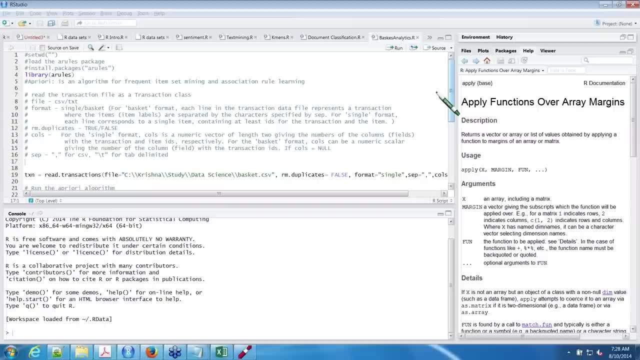 of comments. Once you start working on a single technology for years, then only you know in and out of the commands. Ok, So when you start working with the data science, you will be working in multiple technology. Sometimes you will be working with excels- few excels also there is- you will be working. 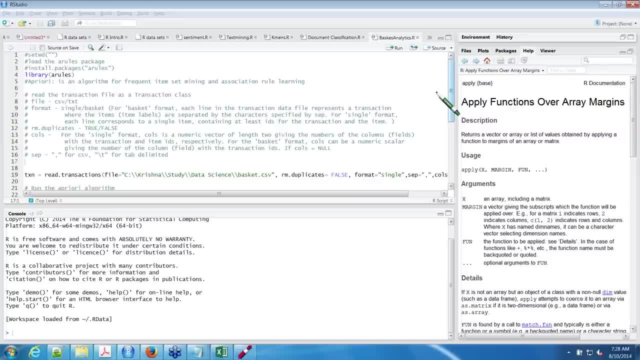 Ok, Lot of calculations also you will do in excels for quick turn around times and as well as you will be working with the java, sometimes with python as well, Ok, Sometimes with R. It is better to make a kind of a document which has a frequent use. 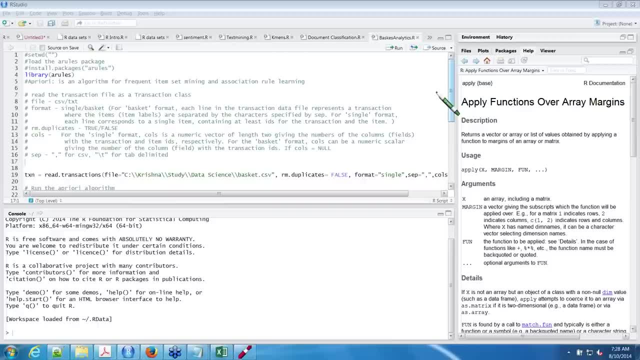 of comments and as well, a kind of a easy access for different models. what are the packages? you want to use it? So that will help you a lot. Ok, Fine, mother. So just we are starting the practicals. just follow on from here. 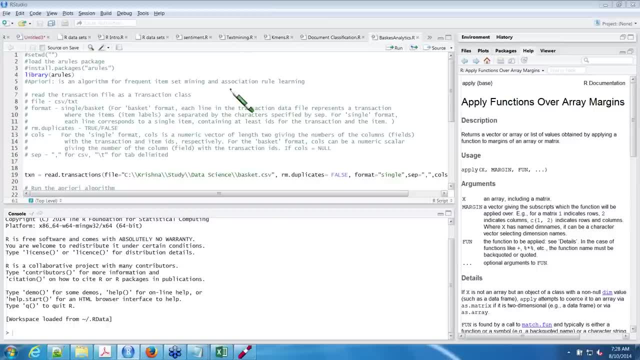 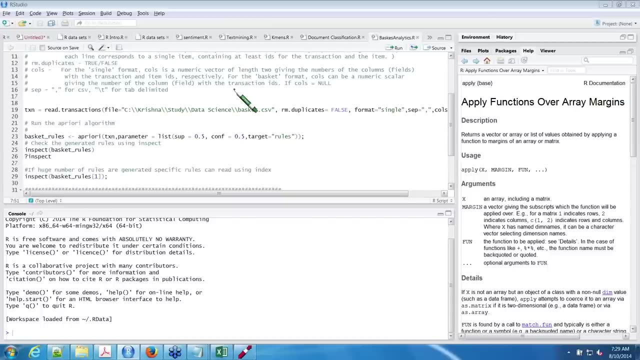 Ok. So, as usual, we have the list of codes for R, and here we are going to use a different types of a package, which is called a rules Ok, Which is called a rules Ok, And under that a rules, we have a functions which is called apori. 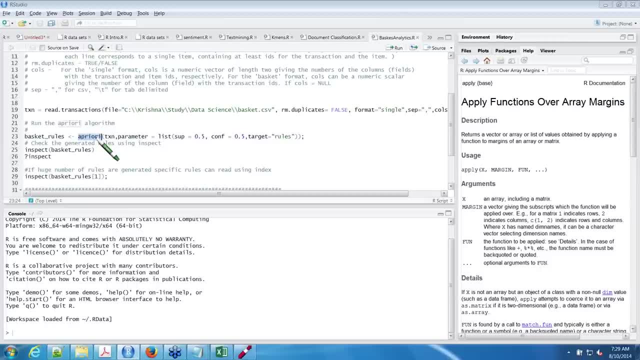 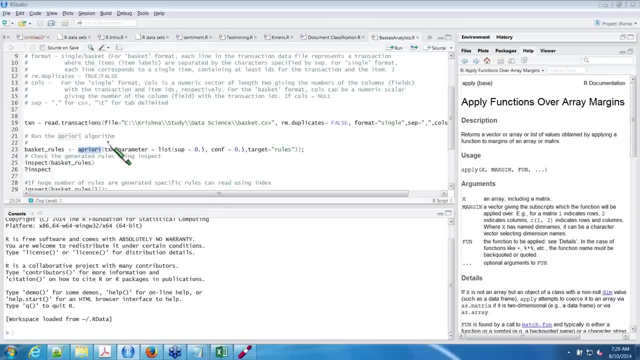 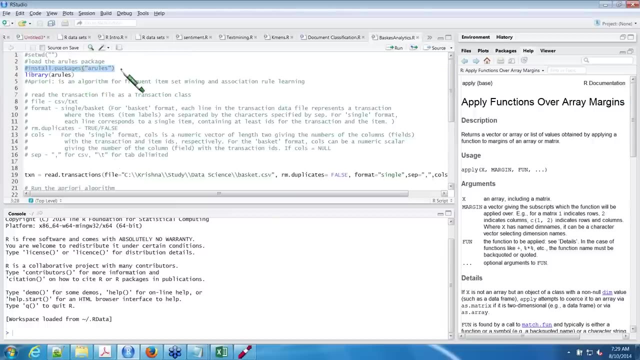 Ok, Where in previous thing we have seen the tfidf function and kmin functions, Here we are going to see the different functions, which is called apori. Ok, So we can install the package If the package is not present in your R and, as usual, we can set the working directly to. 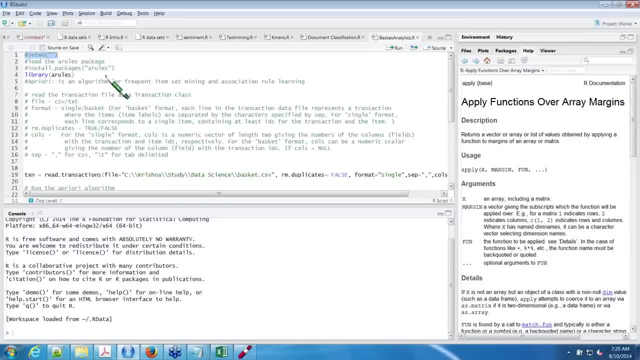 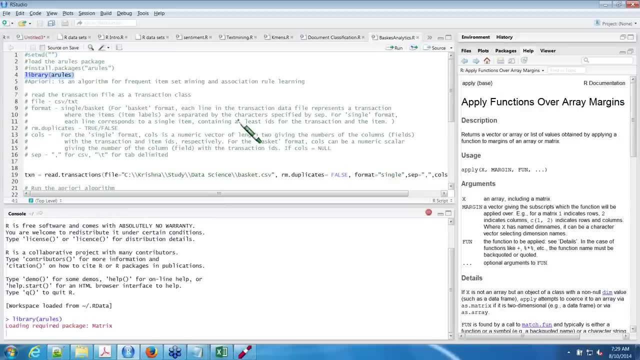 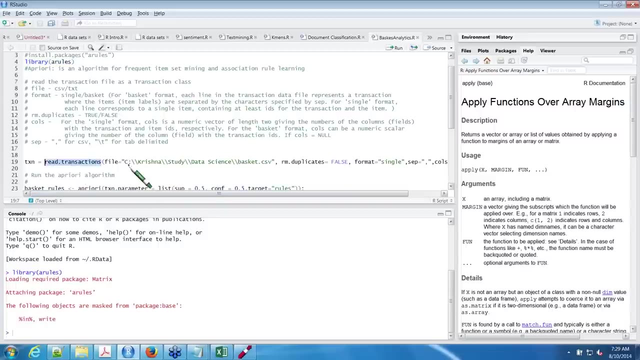 read the data from that particular location and to write the data to particular locations, Ok. So now, previously we have seen read dot, csv, read dot table. to read a csv file, Ok. Or read a csv file or a different separated comma, separated file or different delimiter. 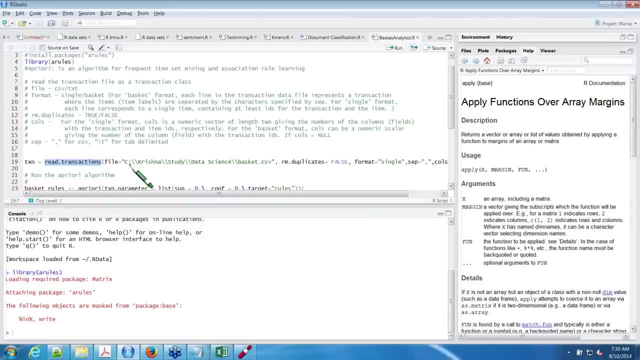 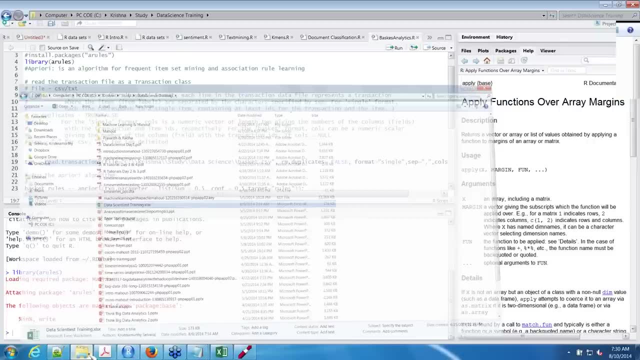 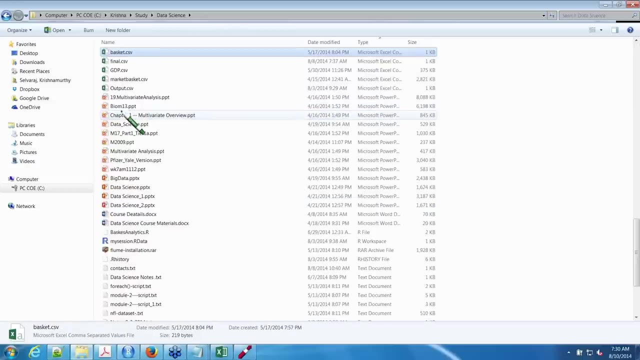 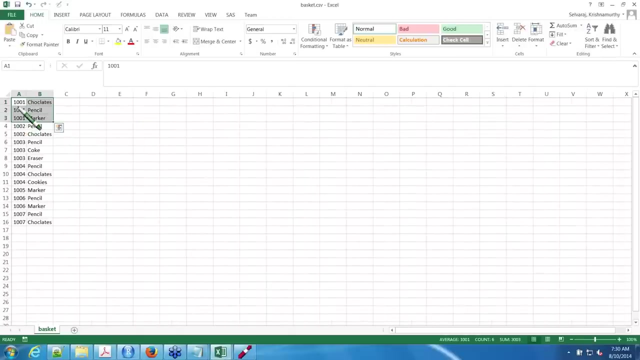 files. Now we have a mechanism is called a transaction, and the file should be in this format only. Ok, Transaction id are the products. So first column should be a transaction id and second column to be a products. So this is how it should be. 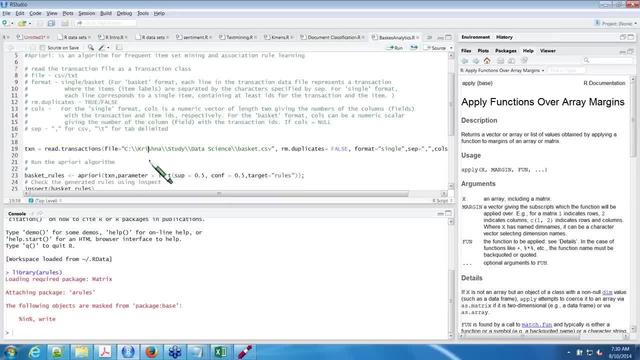 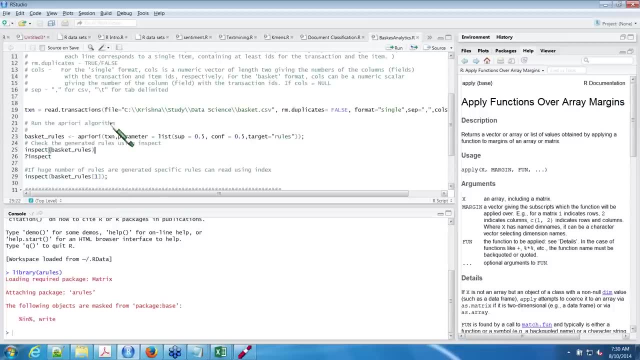 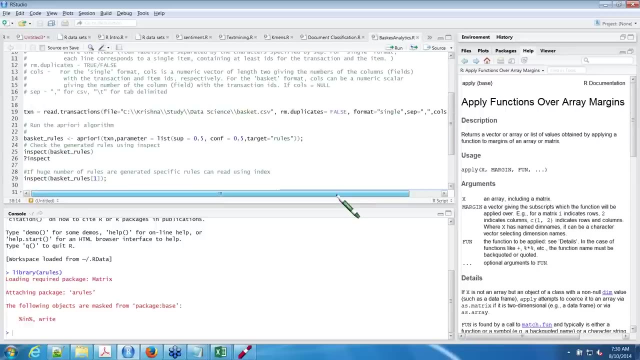 Ok, So now? So I am going to read the transaction: Remove duplicates is equal to false. If any duplicates is there, don't remove it. And format is equal to single and separated by comma And columns is equal to first column. 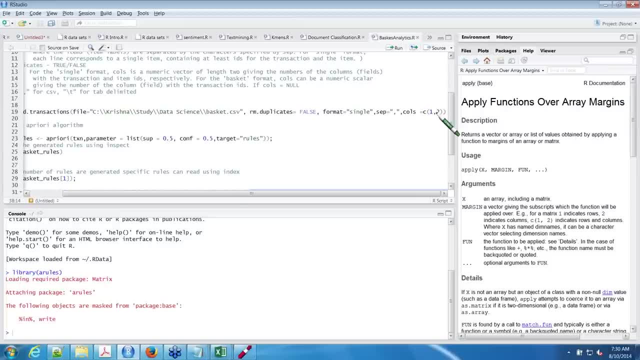 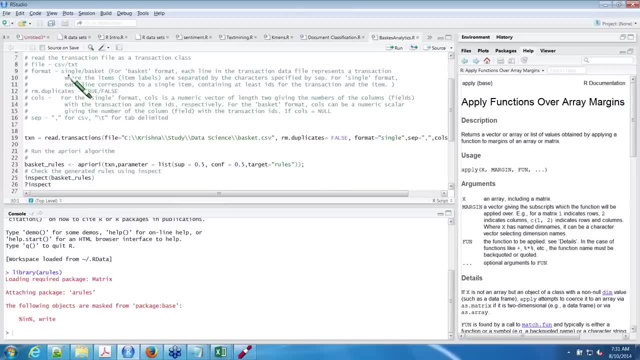 Columns is equal to first and second column. The format is equal to single. Ok, What it means is like it's a single basket. It's a single basket where you have all the transaction which is present in transaction id and the kind of products in the file. 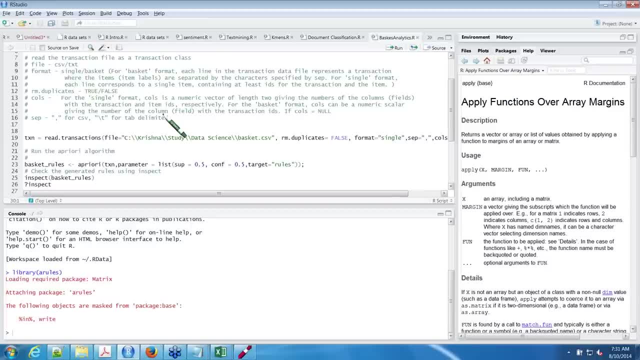 So that's the meaning of it. It is single. Ok, So where each line will have the transaction id and the product name, that is called single. Here we are not require customer id. We are not going to profile them and not going to analyze based on the customer id. 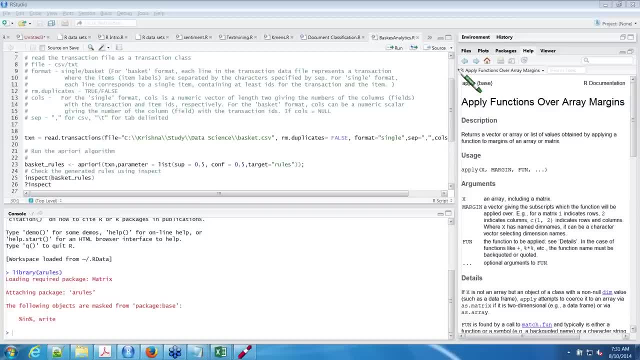 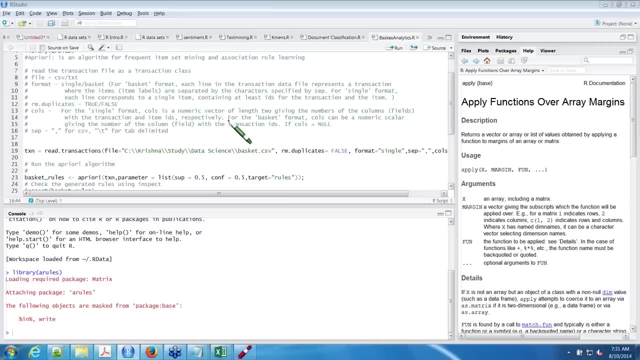 It's only a market basket analysis. It's not based on customer Finds in the Ok. So now This reader transaction will read the data set in the form of a transactions, Because Aporia understands only a transaction data. 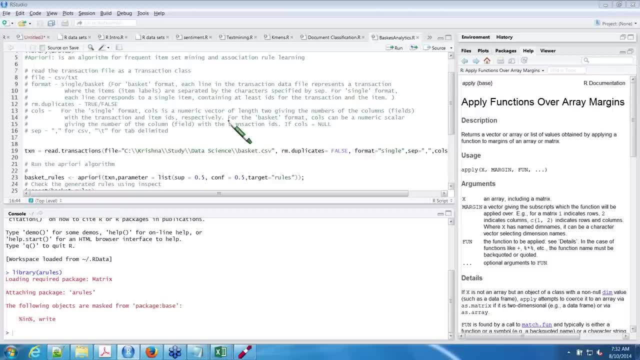 It does not understand the CSV file, Normal data frame. it does not understand It will be in the form of a transactions. So when you read this data set: Ok, We have seven transactions. Previously it used to get the seven rows: number of rows. number of columns. 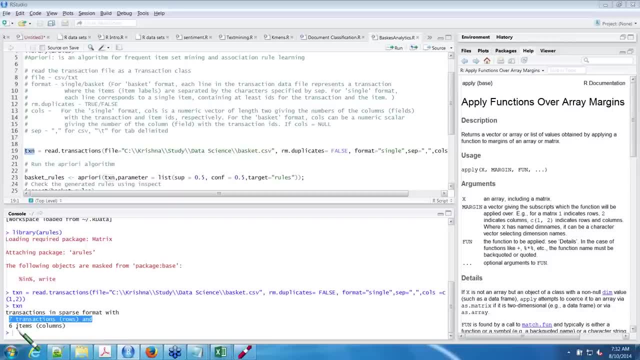 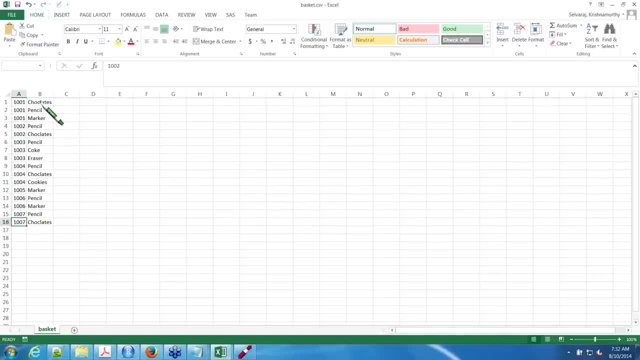 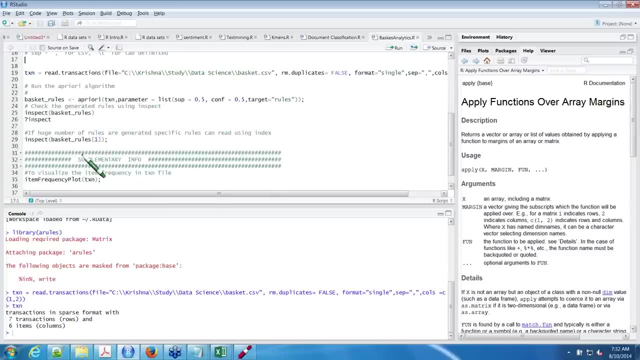 If you look at the transaction, Seven transaction has been done and six items purchased- Seven transaction. If you take a uniqueness of this, it will be a six products purchased. So now I am going to apply to the Aporia model. 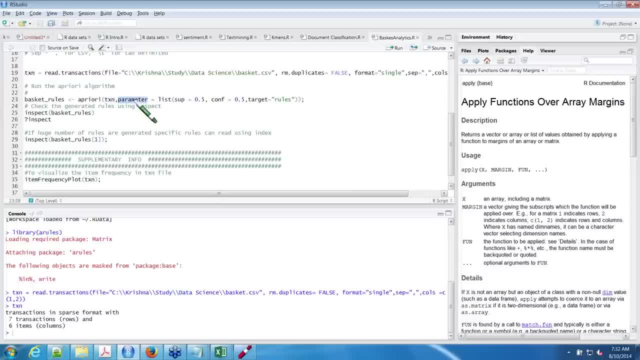 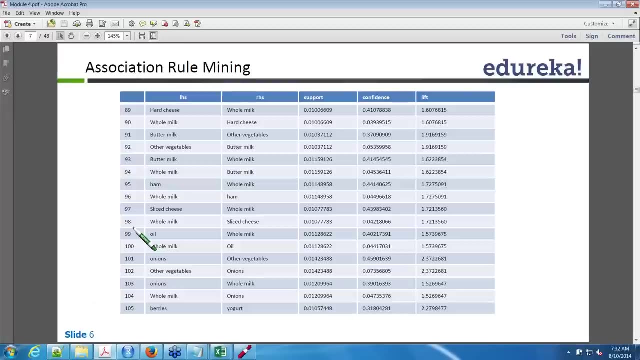 The input is going to be the transaction and I am going to have a parameter called support, confidence and target is going to be the rules. So what is the support and confidence? Ok, The support and confidence. So, if you look at this, 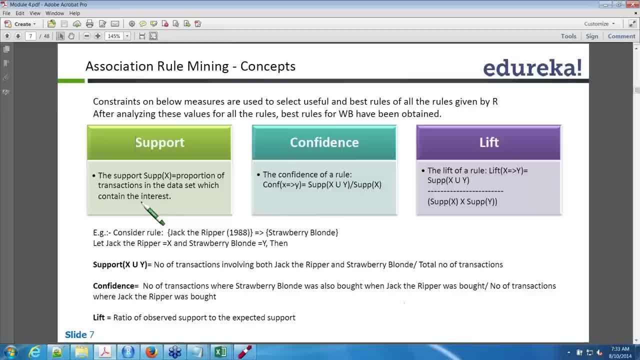 Proportion of transaction in data set which contains Which contain the interest, Which means To what portion of a data The product should be present in the transaction. For example, Today I made another transaction In that only one time One product is coming. 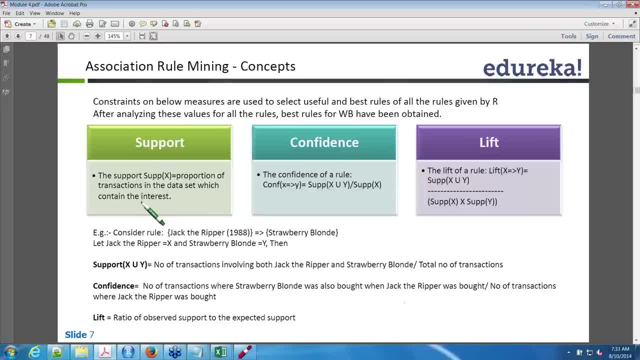 So that product I cannot use for my analysis, At least minimum, what level of percentage a product should be present in all the transaction? That product only will be considered for the association rule mining. That is called support And confidence. Ok, Number of transactions. 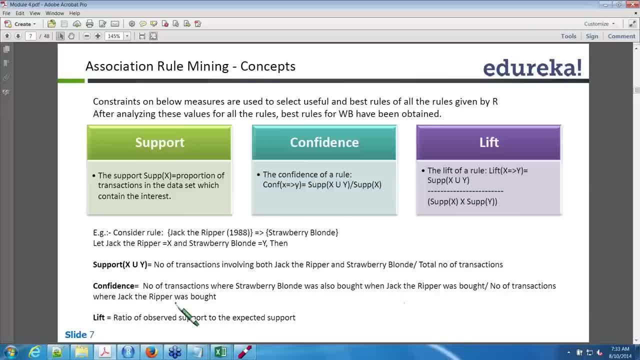 Divided by That is To what level of total number of transaction. For example, A product is coming 10 times, But the total transaction which is happened on that day is 1000.. So which is 10 by 1000.? 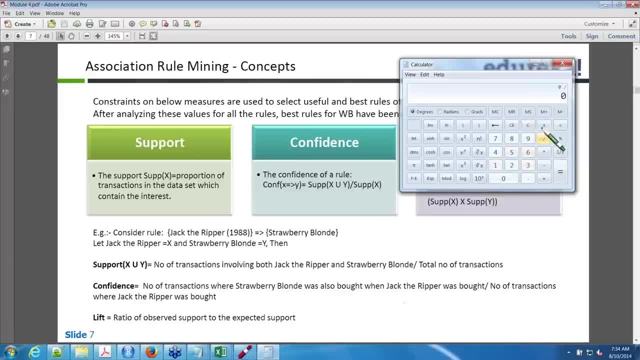 Ok, So if you look at 10 by So, only 0.01 percentage, Only 0.10 percentage of a product is present in total of transactions When compared with the another product. So to what level of confidence? 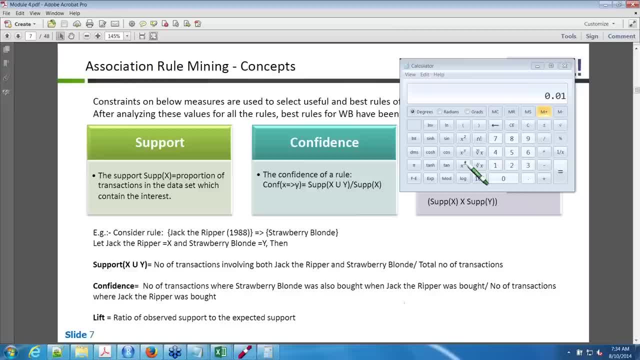 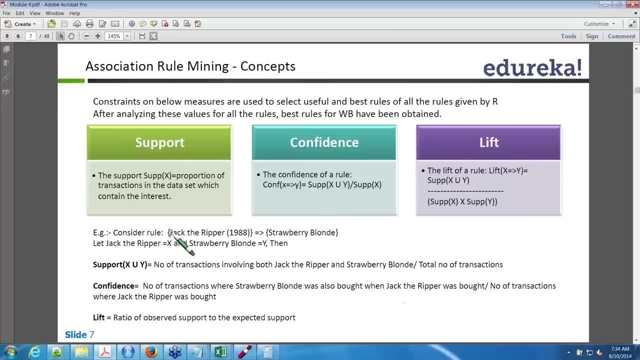 For a product to be present Which I have to take into account for my analysis. So if you look at the examples, So take an examples, Two examples, So: Jack the Ripper and Strawberry. So which means Whenever the Jack the Ripper is buyed. 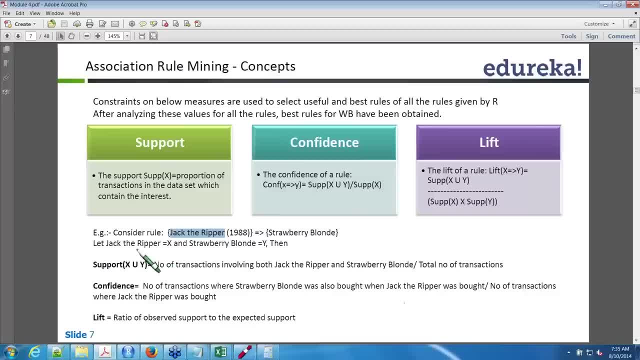 Strawberry Blonde is also buy together. Take Jack Ripper as X and Strawberry as Y. Number of transaction involving both Jack and the Ripper- Jack, Ripper and Strawberry- Divided by total number of transaction- will be the support. Ok, So what level of percentage it should be present? 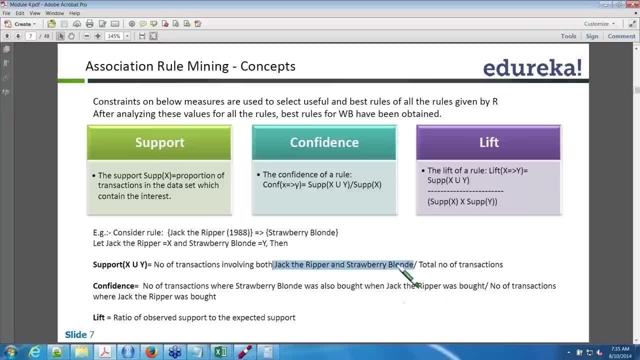 So that This product are purchased together And we have a balance And we have a minimal number of transactions Which I take into account for my analysis. So once again I am explaining Number of transactions involving both the products purchased together. 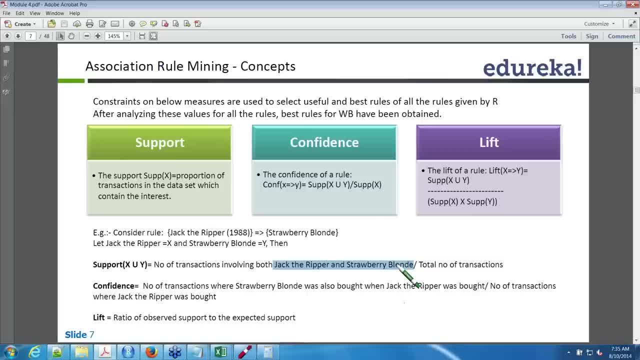 So what are the transactions? Number of transaction: A purchase of both shampoo and air conditioner together Divided by total number of transaction. So that should be minimum of 50 percentage For me to consider that basket, Else I will not consider that basket. 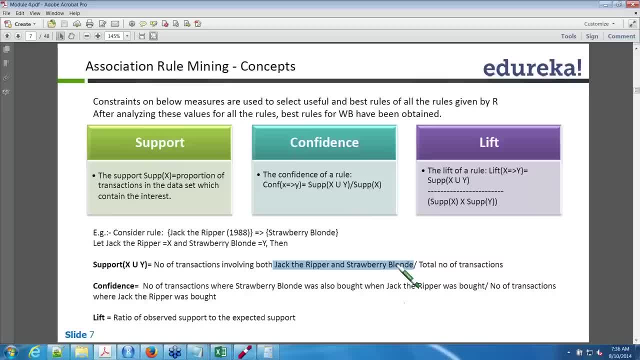 So what extent I should be considering is what called support And confidence: Number of transaction Where Strawberry Blonde was bought When the Jack was bought, Divided by number of transaction where Jack the Ripper was bought. So this is: 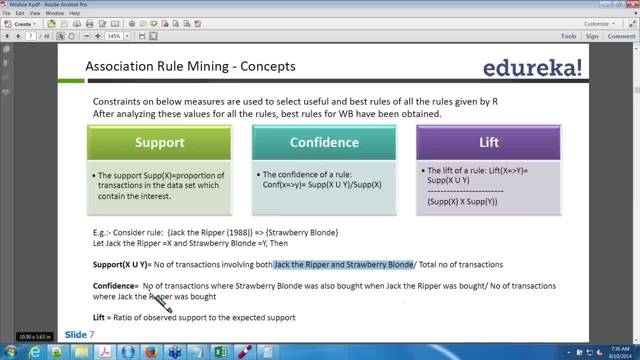 To what extent of a relationship between the two products Divided by The number of transactions of the primary product. So when I say primary product, Whenever for any product You will have a primary Based on that primary only you will add the child products to that. 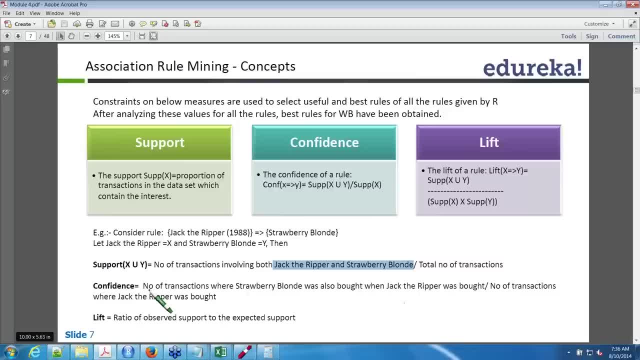 So you will not buy a peanuts Because of peanuts. you buy a beer. No, You buy a beer Because of that, only you buy a peanuts. So to what extent of weightage the primary product is got. So that is called confidence. 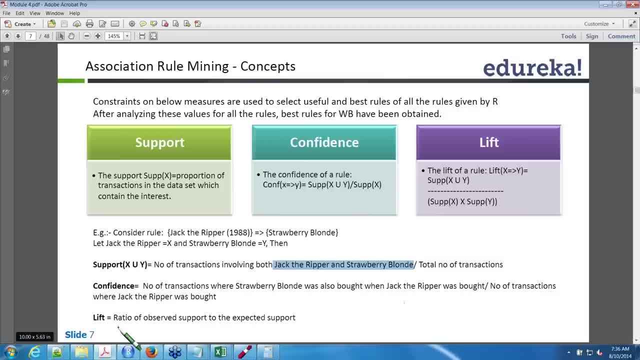 So when beer is buy, I am very confident that peanuts will be buy together. So that level of percentage is called the confidence. Is it clear? R stage is clear Between support and confidence. only the denominator is different: Yes, No. 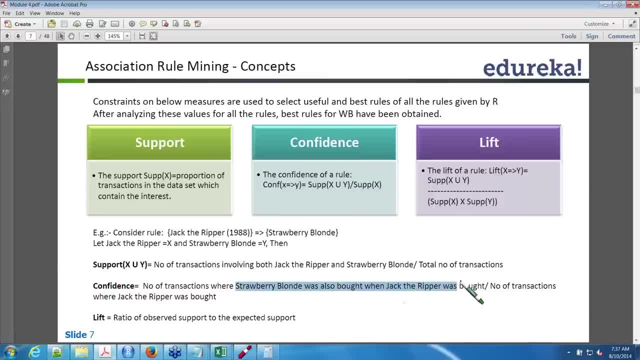 It is reverse Here. it is reverse. Okay. Here Jack the Ripper and Strawberry are becoming like a SuperVisit Linux. Okay, It is not a supervised learning. Okay, It is finding out between the two variables. No, We will not give the two variables. 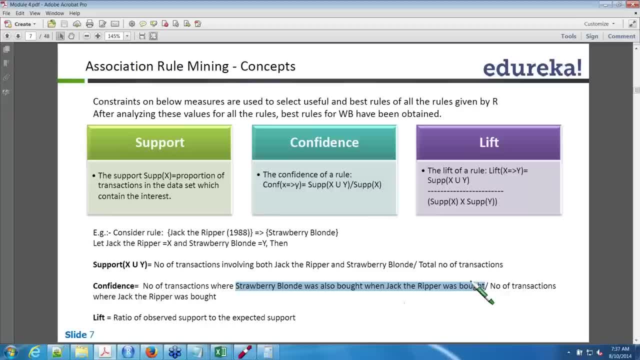 Automatically the system takes Okay And fine, Fine. bizarre. Acceptable confidence level is 50 percentage, So it is as we decide, based upon the number of data, So data science. there is no fixed rules as such. So the minimum what we can have is a 50 percentage. 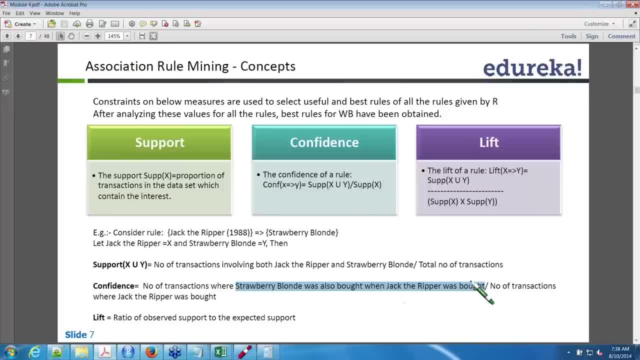 Okay, And to get a better accuracy and to promotions, to be fine, people can have 80 percentage as well. Okay, Fine, Anup And Sundar, How to differentiate numerator in support and confidence. Okay, I will give that Okay. 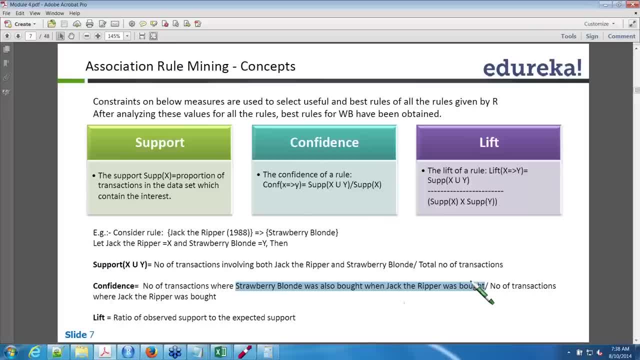 So we will see that. So Y is into X, U. It should be X intersection, Okay. So it is union of part, It is not an intersection, Okay. So why is this? because where, when the Jack is was bought, was also bought this strawberry. 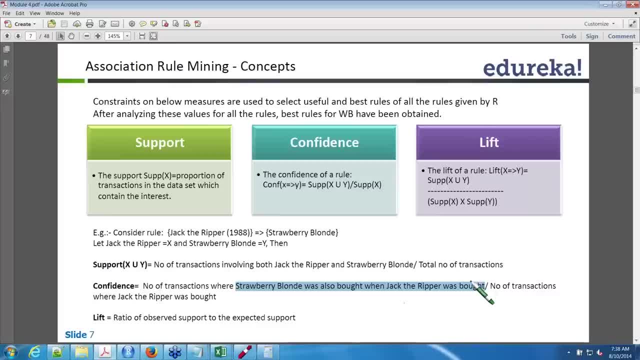 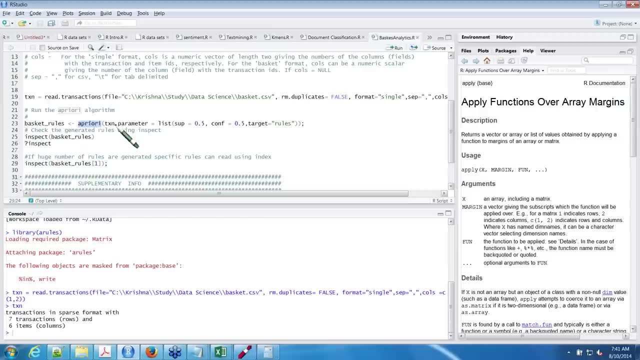 So that is the meaning of it. So there comes the union. So this is the formula for confidence. Okay, So now, if you look at the appory, the parameter is going to be support. I am making as 50 and 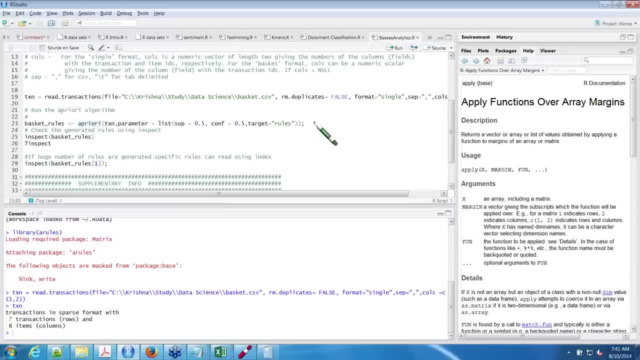 confidence. also, 50 percentage. 0.5 is equal to 50 percentage and target is equal to rules, which will give me a set of rules on what basis your product X is bite with Y. So that is a kind of a rules I will be getting out. 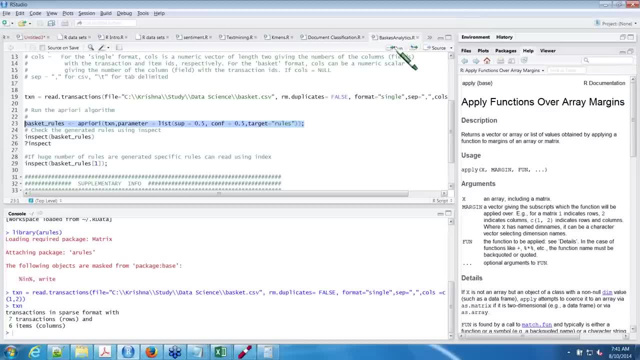 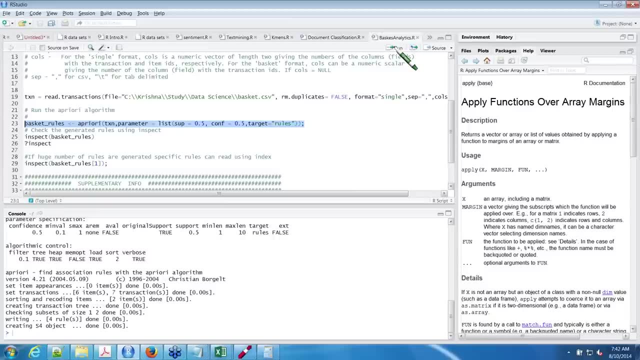 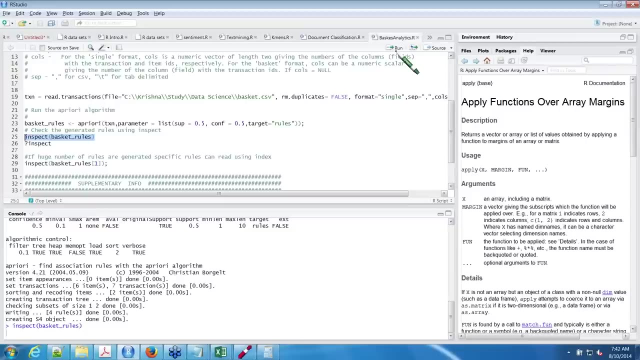 So if you run this, So now I will be getting a certain association. Okay, So I am getting a certain association rules between each and every products. Okay, So if I instruct the rules, it says it is called left hand side and right hand side. 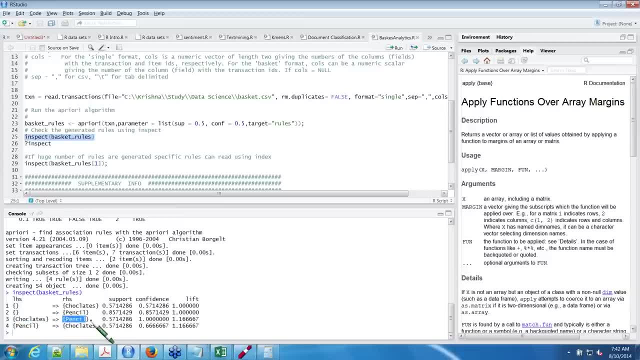 Whenever chocolate is bite, the pencil also bite, together with a 57 percentage of confidence, 57 percent of support and under percentage, it is confidence. where chocolate and pencil are bite together. Whenever a pencil is bite, that is a primary product and the chocolate is bite, it is 57. 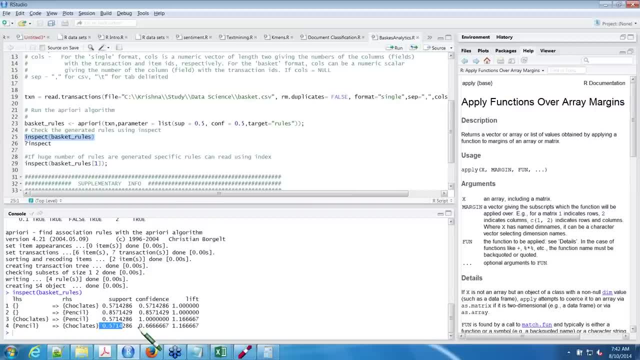 percentage confidence and 0.6, that is a 66 percentage of confidence and 57 percentage of support, Got it- And a lift of 1.16 percentage, that is a increase between this and this. So, which is an observed and expected, can rise. 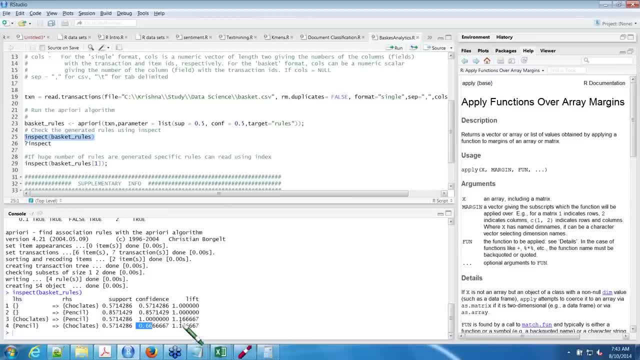 So the lift is only a kind of a information, which is not used for any analysis. The main purpose is support and confidence only. Okay, So that is how you determine what level of product and which are the products is purchased together while- and then what are the products can be put together for a promotions. 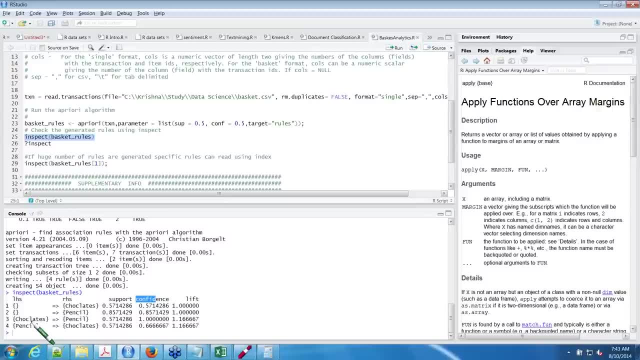 So one product you will promote, which in turn The sales into a sale of multiple products. That is the main objective of this market basket analysis. Okay, How does the retransaction function understand first column transaction ID or is the transaction always? is transaction ID to be always first column? 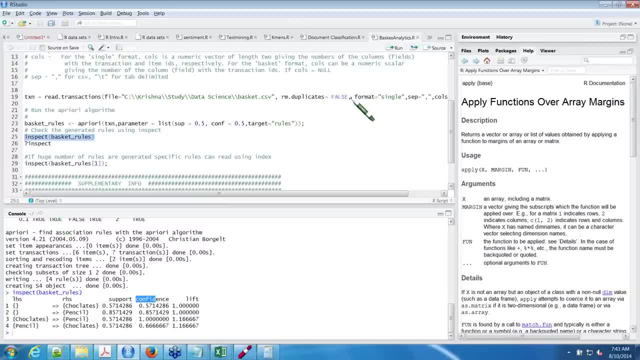 Okay, So that is the reason we are saying it is a single, So which means the data set should be in this form of transaction, ID comma the products. So we say 1 comma 2.. Fine, Fine, Fine. 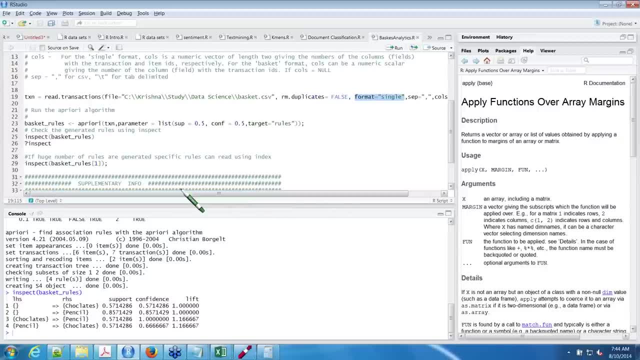 What did you mean when you put 0.5 support and confidence? It is a natural language. Okay, It is 50 percentage, Fine, and all At least 50 percent of a product should be always buy together and conference also should have 50 percentage. 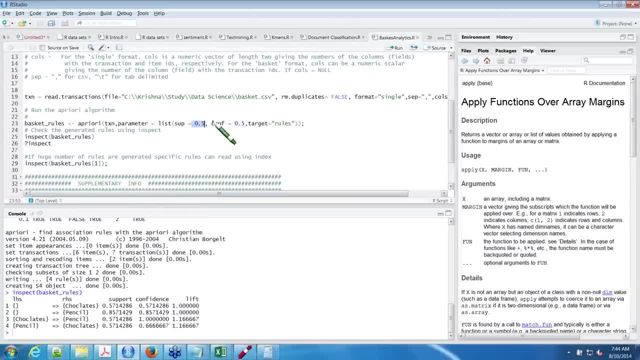 Okay, Okay, so it's our mechanism. it's not fixed, so, based on analysis, you can also increase to 80% or 90%. how will you have to determine which are the majority of the products to be purchased or put together? so that's the main objective of this. it's as decide based. 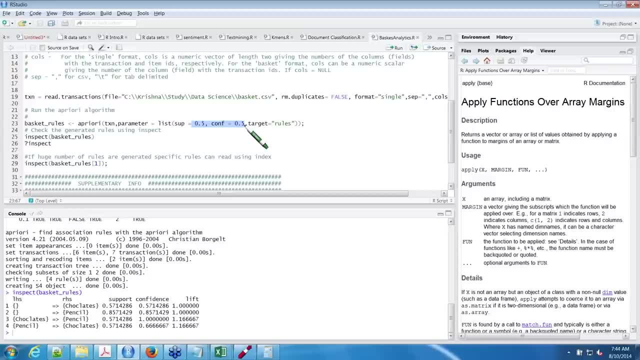 upon seeing the data and how will you want the accuracy? fine, So if it says 100 products you have to put together, I cannot re-alter my retail stores. So majority of things, 90%, I can believe this product will be purchased, then only those. 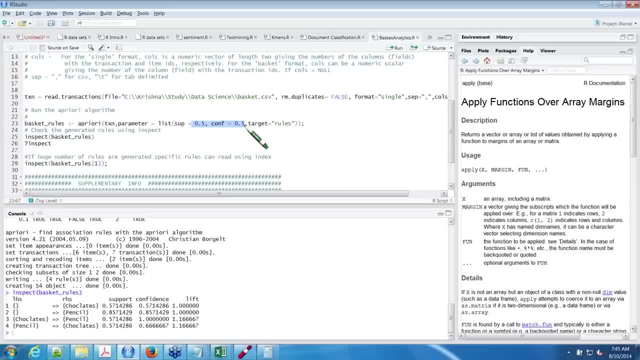 products bring to my attentions, so then you can change it to 0.9,. got it. It is various. it's not fixed. my trial and error method will be changing it. yes, The algorithm will give only the products which falls under this category. 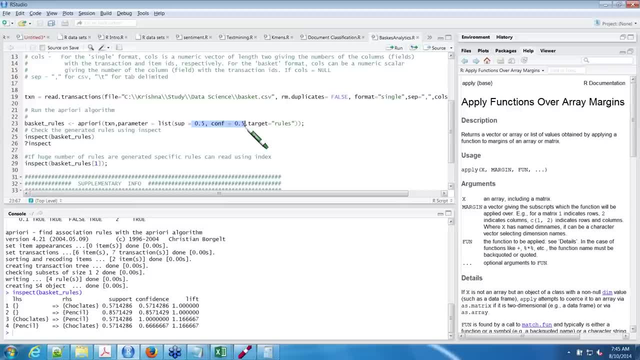 Under this range of confidence and support Other products it will not show. So if you look at the inspect, inspect will give you the rules. So now I am a kind of a store manager. I want to know where I will place my products. so 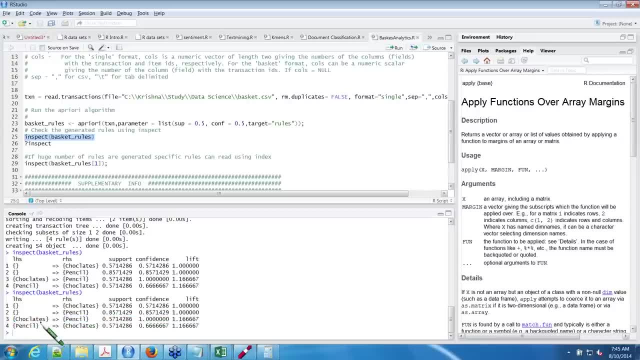 I will place. I bought chocolate and pencils together and I will promote only chocolate. So in this case, 100%. I am confident that whenever you purchase a chocolate, you will buy a pencil together. So in this case, I am 66%. I am only confidence that when you buy a pencil, the buying of chocolate. 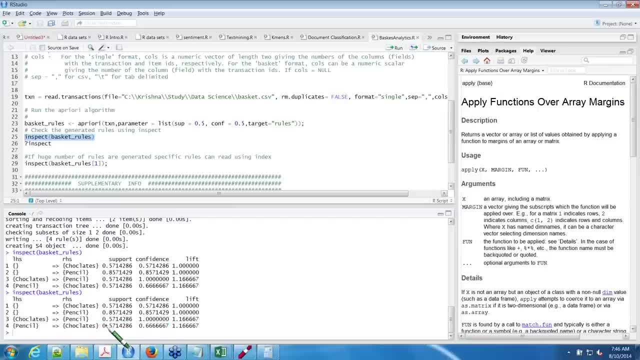 is less, But you can see that 57% of customers is buying pencils and chocolate together. left hand side is going to be the primary product. Right hand side is going to be the final product. 12. the products: the right hand side- the primary product- makes a tense or intense to buy the. 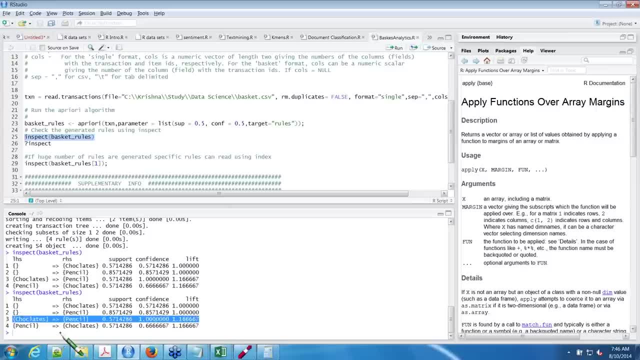 secondary products. so that's the meaning of it. so I will promote only chocolate in turn. it sells pencil, correct, Sundar? is it clear? yeah, can we get the support and conscience for all the products? yes, you make one one our point, or at least one percentage of transaction. 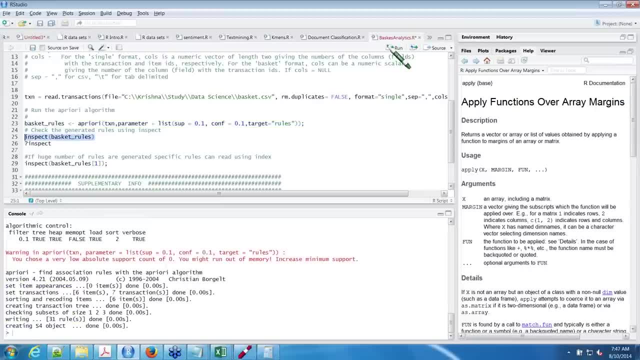 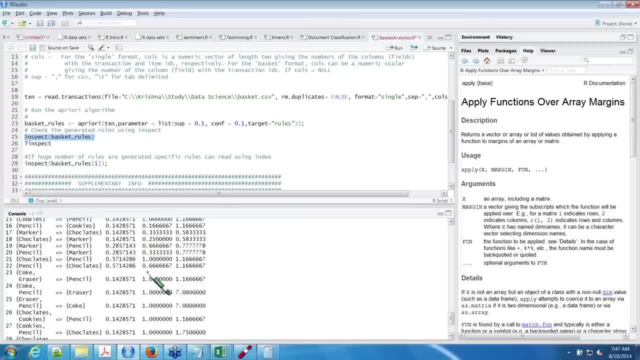 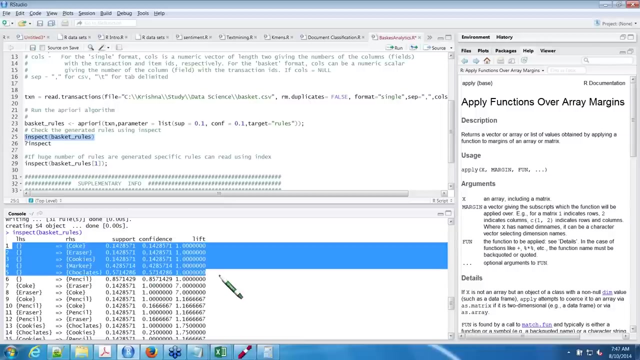 do you see that Coke and a racer by together it is. you see that coke and eraser by together it is 14%, and eraser and coke purchase is only 14% of support. coke, pencil, pencil, coke, eraser, pencil, fine arrow, so the empty is, it is not able to calculate. 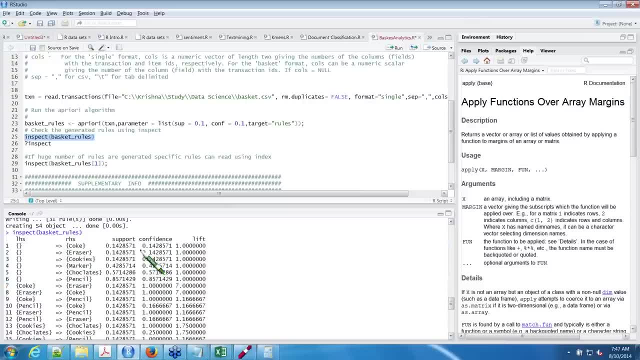 So those data's are. primary product is not determined because if you look at the conference is very less. you see that 0.14 is the conference, Fine arrow and 0.14, you see that it is 0.14, support attribute. you have to look when the 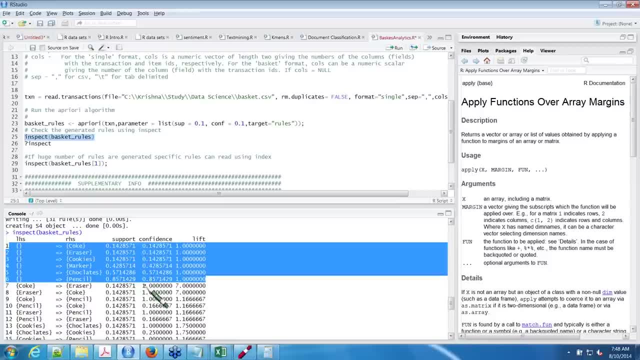 support is there. only you can go for confidence. If the support is not there, It is no point in going for confidence. only 14% of transaction, which is having the combination of products purchased together. the primary weightage will be given to the support only. 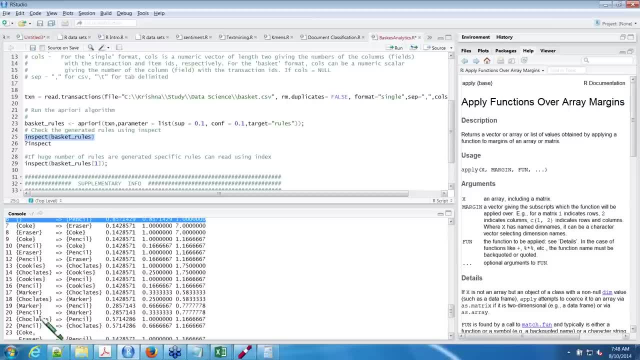 more than the support. so 28%- only pencil and marker is buy together. So I don't want to concentrate on the 28% of customers, I want to concentrate on 57% of customers. what is buying that? only I will concentrate, then only I will look for what. 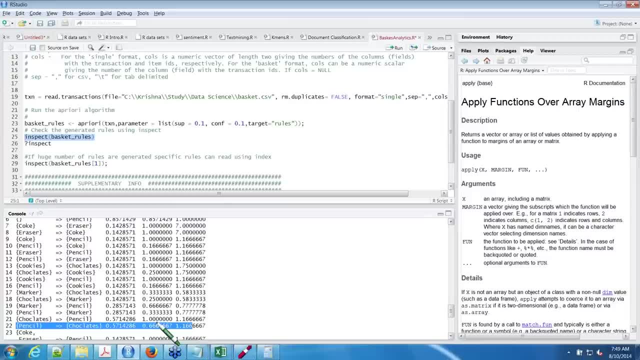 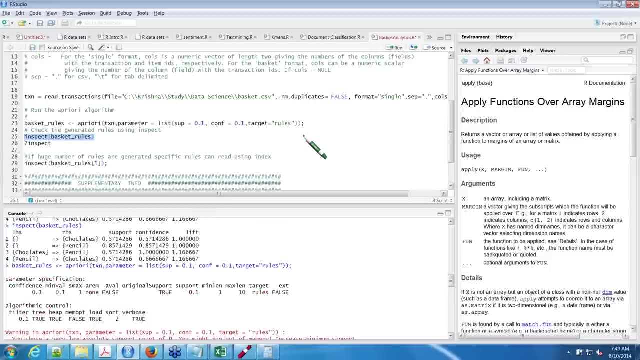 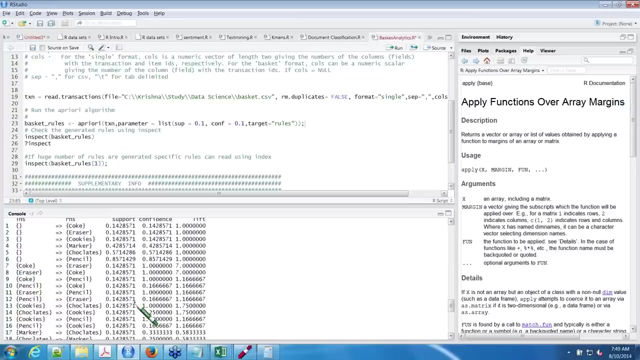 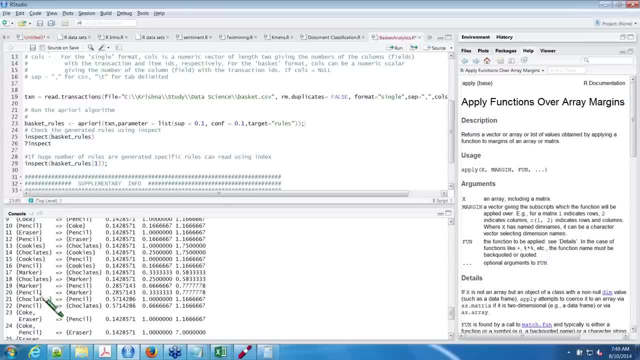 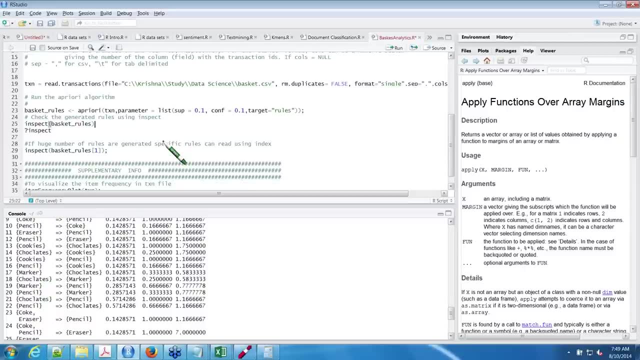 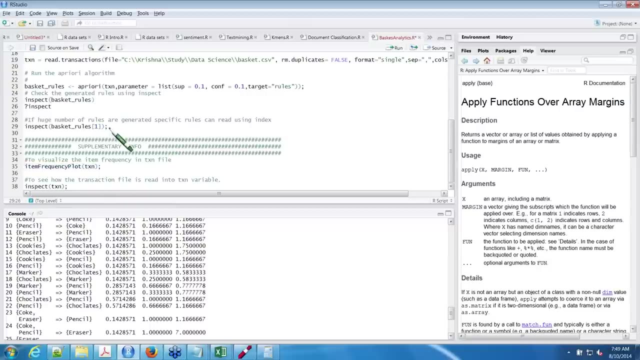 Transactions are more. What is the combination of products buy together? also, it matters. got it ok? So this is the plot. so this is for checking only first product. this is for checking in a plot. You can check in a graph. 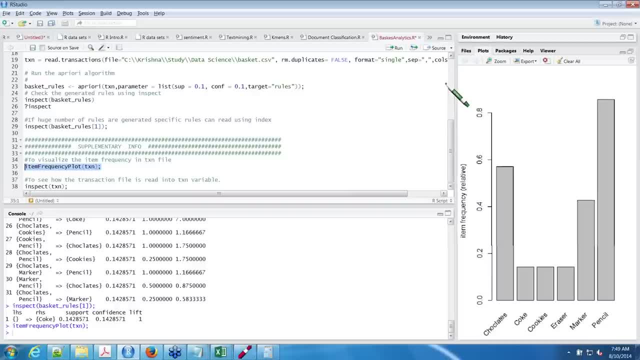 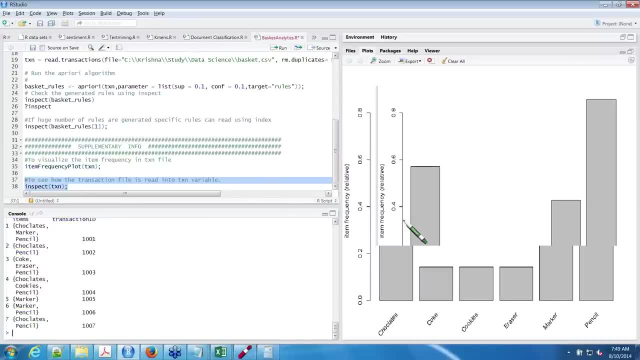 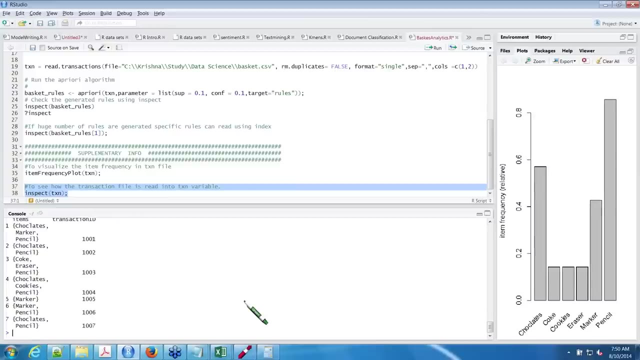 Ok, In a graph, visually. that's all. So this is to inspect the transactions. So we have read the transaction right. this is how the transaction will be converted. For item one, transaction one, it converts into an array of, that is, a vectors of the. 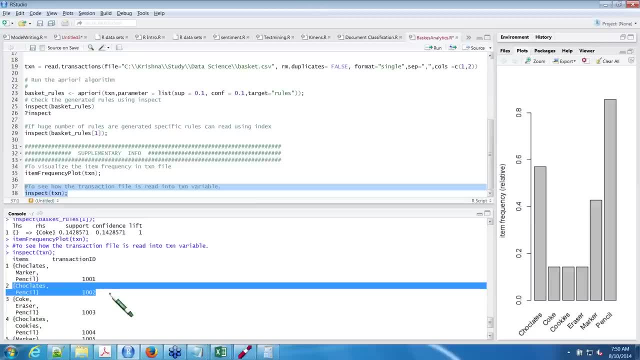 products purchased, Find bin. so this is how it converts. you see the transaction items. so the first column should be always a transaction, second column to be a list of products. Then it converts into a list of vectors for each product. what is the each transaction? 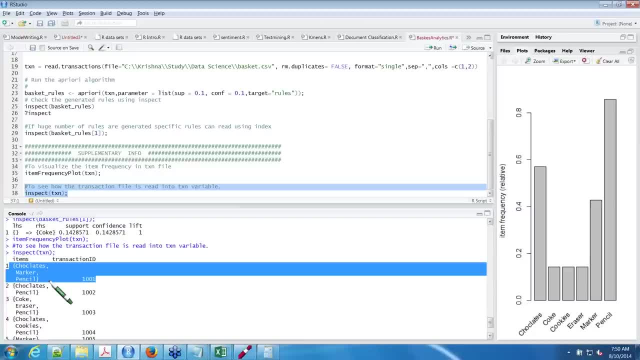 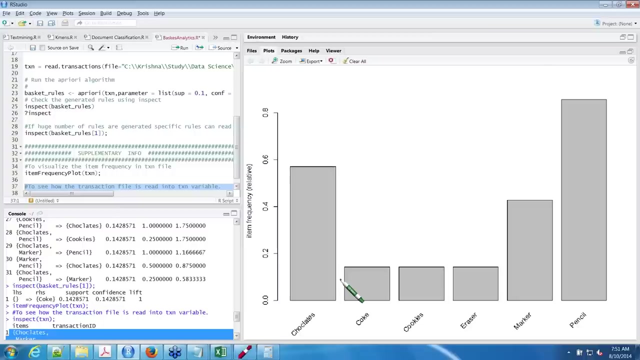 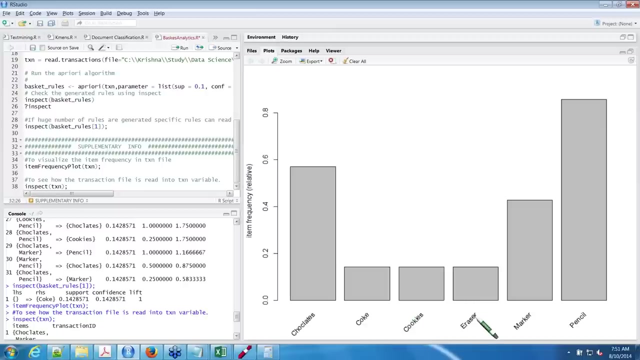 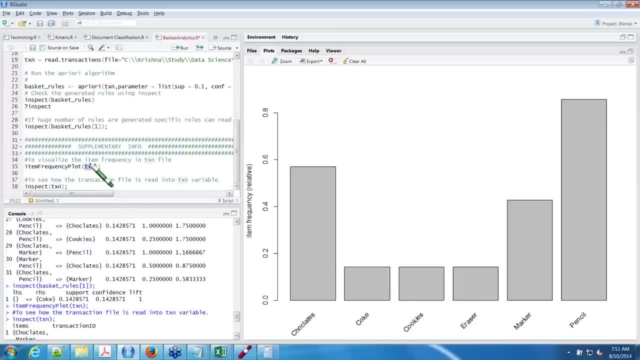 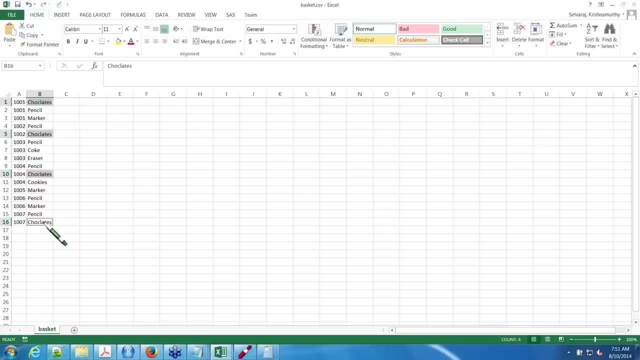 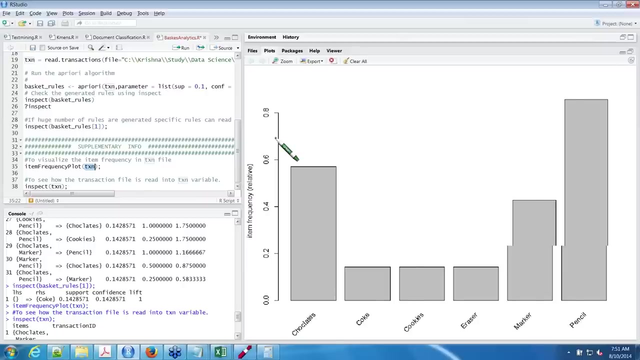 is the count in the transaction. so in the transaction, just if you go here so count of this one, two, three, four, right? so out of all this transaction, what is the frequency of this transaction? got it? it is four times, when you add everything, the number of frequency. 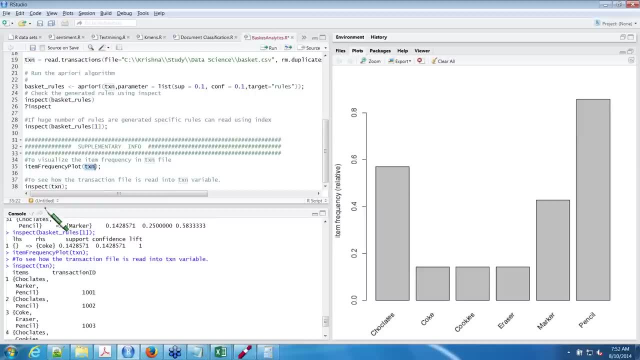 plot. ok, so around sixty percentage Around coke occupies the data of twenty percentage around cookies. twenty, this twenty, but pencil as a frequency of product which is higher when compared to any other product. so that is the meaning of it. fine, Sundar. 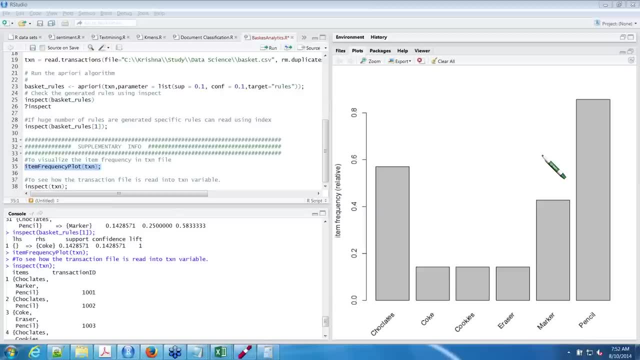 So total number of products. so it is the number of products divided by total number of transactions. No, not a combination. can we say twenty percent is a combination of chocolate and coke? no, it is only each product. how many times is present in the transaction. that's all it. 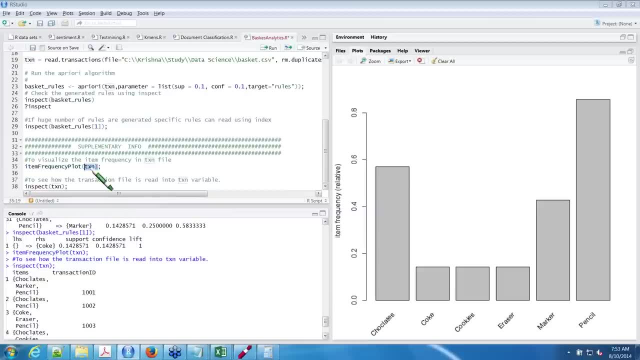 is not a combination. it is only a frequency plot for transaction data, not for the basket rules. ok, so only a frequency plot. so number of transactions divided by the total number of transactions. No problem, Anup, ask many questions, you rise. I welcome that. ok, so I want it to be. 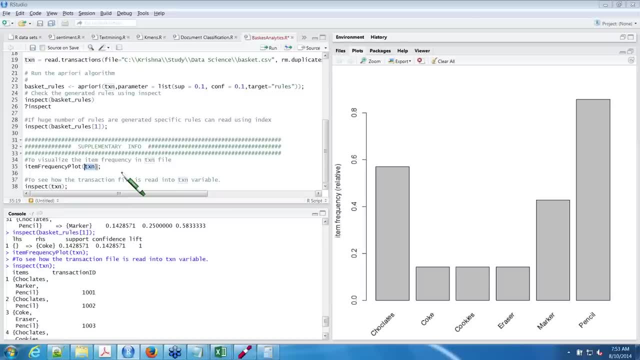 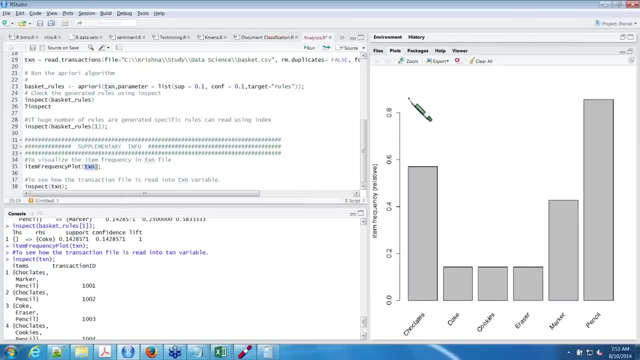 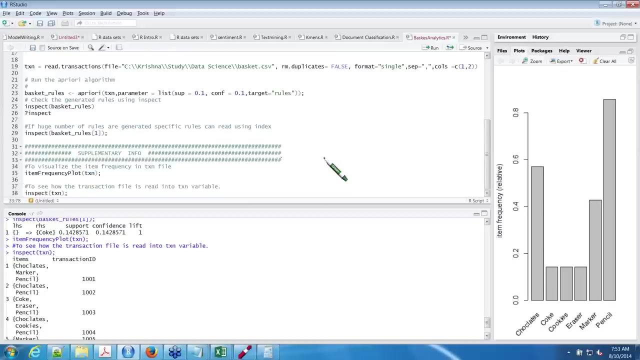 clear. ok, yes, that's for each item. fine, Anup any other questions. if I missed any question, can you retest it please? Ok, Thank you, Thank you. Any remaining questions? No problem, Thank you, Thank you all very much.